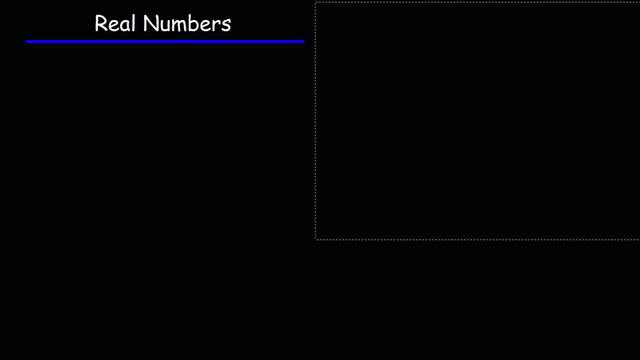 real numbers can be broken up into two categories: rational and irrational numbers. now, before I give the definition of these two, let's talk about the numbers that are included in this category. first we have integers. integers are numbers such as negative three, negative, two, negative one, zero, one, two and so forth. next, 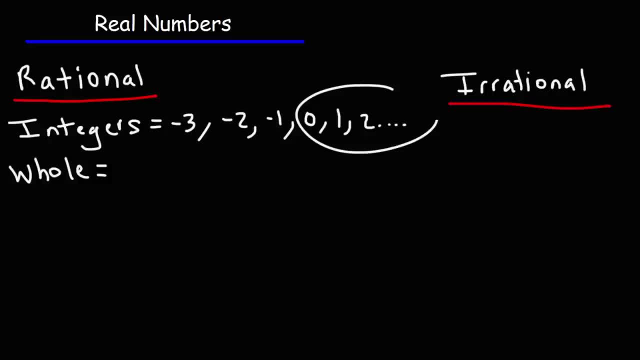 we have integers, and integers are numbers such as negative three, negative two, negative one, zero, one, two and so forth. next we have whole numbers which are integers, starting from zero. so this is going to be zero one, two, three, four and so forth. and then next we have natural. 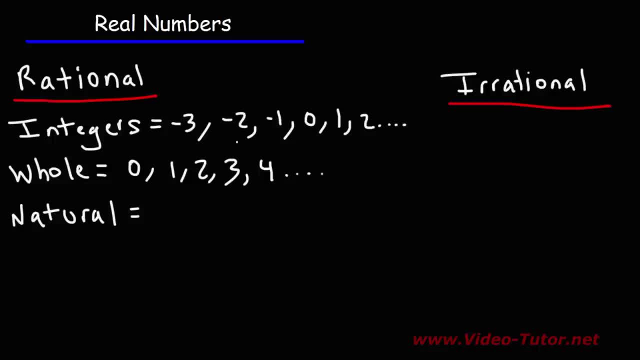 numbers. natural numbers are whole numbers, but starting from one. so one, two, three, four, those are natural numbers. now a rational number is any number that can be put in a fraction, let's say a or b, where both a and b are integers. so three over four, three is an integer, four is an integer, three over four is a. 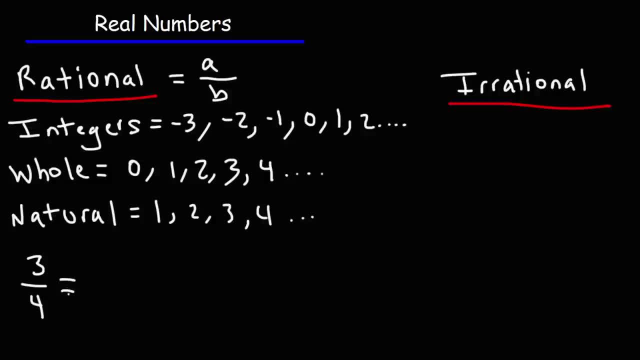 fraction, and that is a rational number. three over four is point seven. five as a decimal number, point fifteen. this is a rational number because you can express it as a fraction using integers. point 15 is 15 over 100 and you can reduce that if you divide both numbers by 5. 15 divided by 5 is 3, 100 divided by 5 is 20. so 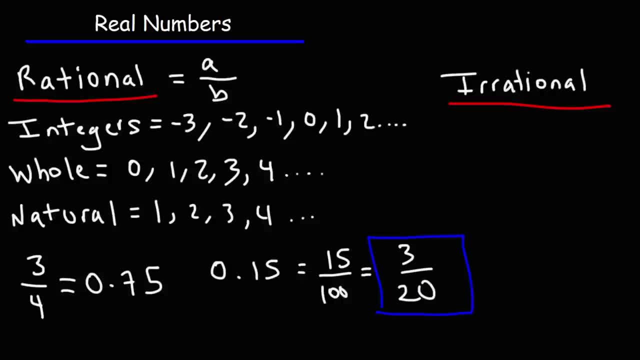 point 15 can be reduced to 3 over 20, which means point 15 is a rational number. we can write it as a fraction of two integers. now let's talk about why home numbers, natural numbers and integers are rational numbers. remember: a rational number is any number that can be put as a fraction using two integers. so the 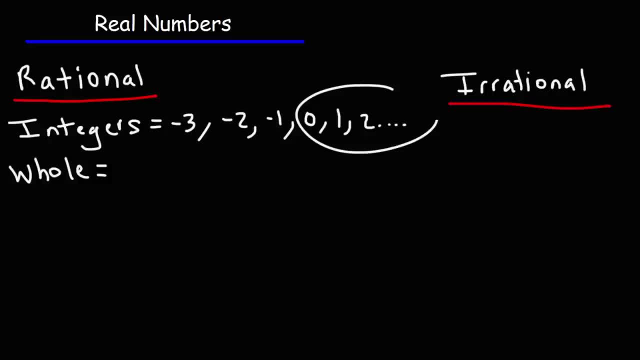 we have integers, and integers are numbers such as negative three, negative two, negative one, zero, one, two and so forth. next we have whole numbers which are integers, starting from zero. so this is going to be zero one, two, three, four and so forth. and then next we have natural. 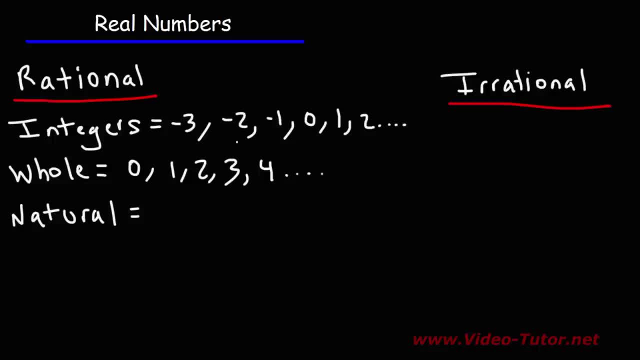 numbers. natural numbers are whole numbers, but starting from one. so one, two, three, four, those are natural numbers. now a rational number is any number that can be put in a fraction, let's say a or b, where both a and b are integers. so three over four, three is an integer, four is an integer, three over four is a. 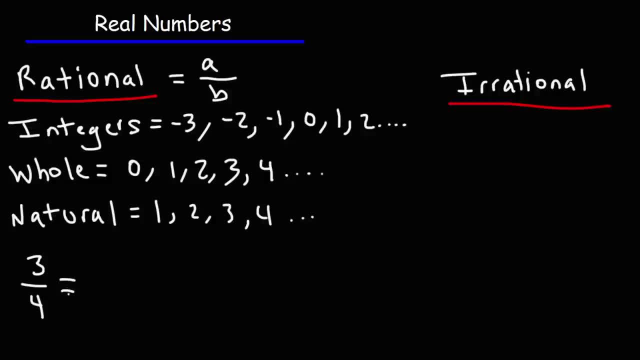 fraction, and that is a rational number. three over four is point seven. five as a decimal number, point fifteen. this is a rational number because you can express it as a fraction using integers. point 15 is 15 over 100 and you can reduce that if you divide both numbers by 5. 15 divided by 5 is 3, 100 divided by 5 is 20. so 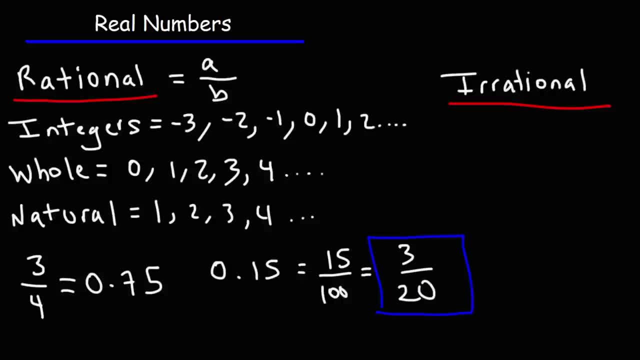 point 15 can be reduced to 3 over 20, which means point 15 is a rational number. we can write it as a fraction of two integers. now let's talk about why home numbers, natural numbers and integers are rational numbers. remember: a rational number is any number that could be put as a fraction using two integers. so the 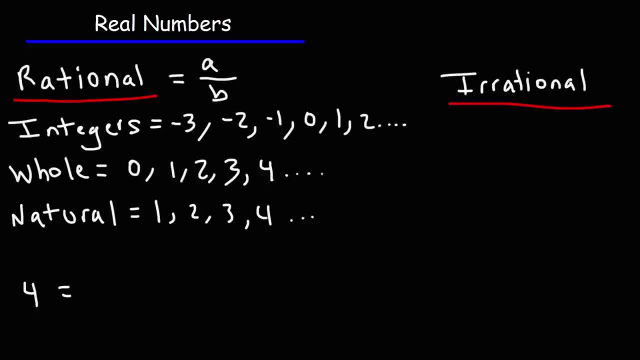 natural number 4. why is that rational? well, we can write 4 as a fraction of two integers. 4 is equivalent to 8 over 2. think about the integer negative 3. we can write that as a fraction of two integers. we could say this is negative. 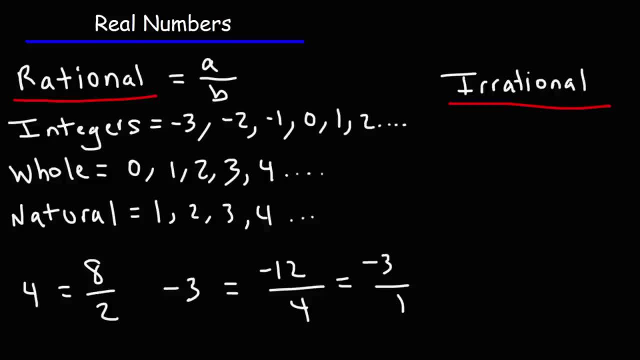 12 divided by 4, or we could say it's a negative 3 over 1. so all of these numbers, whole numbers, natural numbers, integers. you can put them into fractions using integers, which makes them rational numbers, and everything that we've considered on this side so far are real numbers. so now, 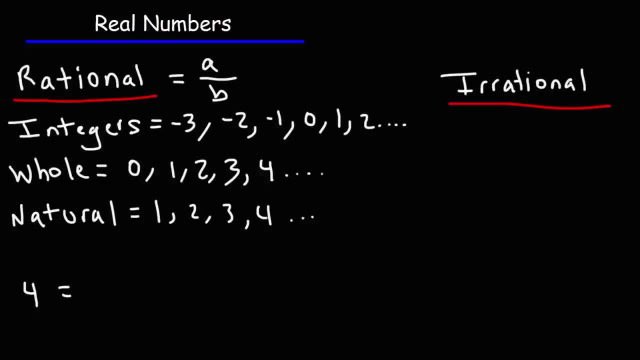 natural number 4. why is that rational? well, we can write for: as a fraction of two integers, 4 is equivalent to 8 over 2. think about the integer negative 3. we can write that as a fraction of two integers. we could say: this is a. 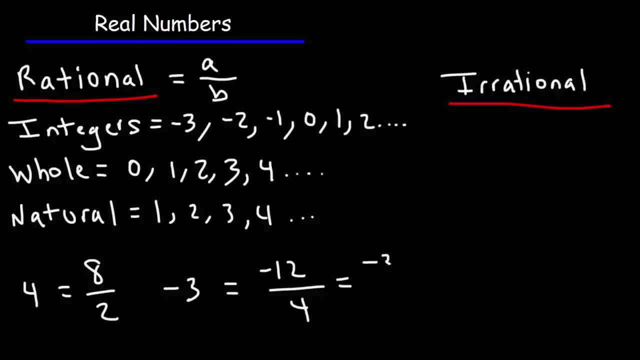 negative 12 divided by 4, or we could say it's a negative 3 over 1. so all of these numbers- whole numbers, natural numbers, integers- you can put them into fractions using integers, which makes them rational numbers, and everything that we've considered on this side so far are real numbers. so now let's talk about the. 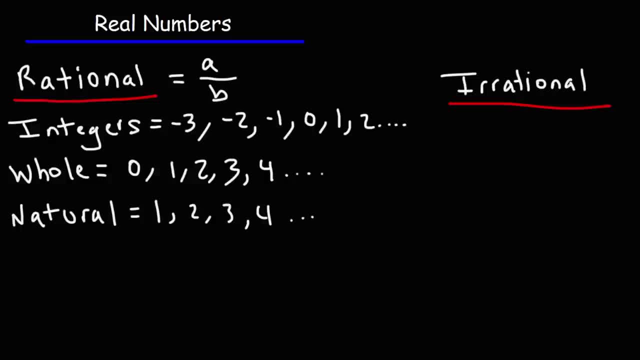 other half of real numbers, that is, irrational numbers. an irrational number cannot be put in a fraction of two integers. so, for instance, the square root of 2, this is equal to one point, four, one, four, two, one, three, and it goes on forever. you can't write this number in terms of two integers using a fraction. 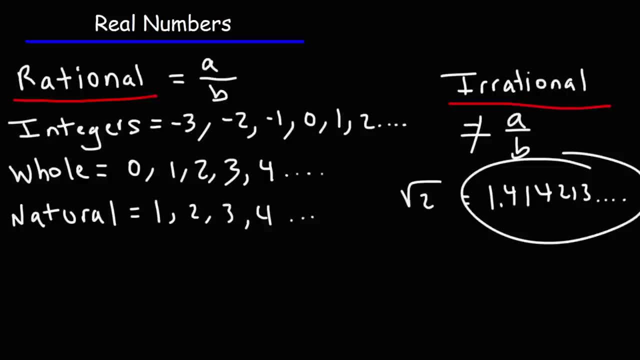 you can't write this number in terms of two integers using a fraction irrational numbers. they tend to be non-repeating decimals and they are non-terminating. they go on forever. you know what? let's write that down so: non-repeating and non-terminating decimals. 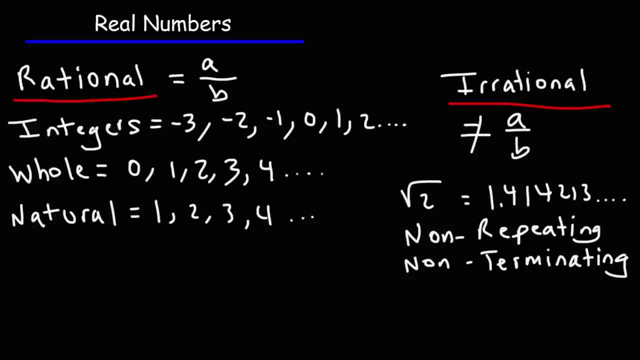 another example of this is the number e. if you type in e in your calculator, you'll get two point seven, one eight, two eight, one eight, and this just keeps on going. so this is an irrational number. it's non-repeating, non-terminating. next we have the number pi. pi is three point one, four, one, five, nine, two, six, and this: 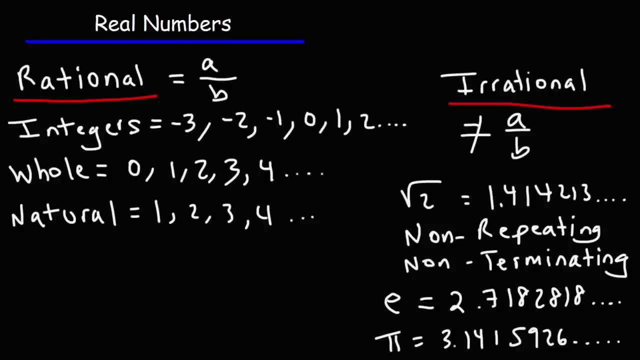 goes on. that's non-repeating and non-terminating, so that's gonna be an irrational number. you can't put pi in terms of, you can't write it as a fraction of two integers. so pi and the square root of two, those are irrational numbers, but they're still real numbers, though you could plot it on a number. 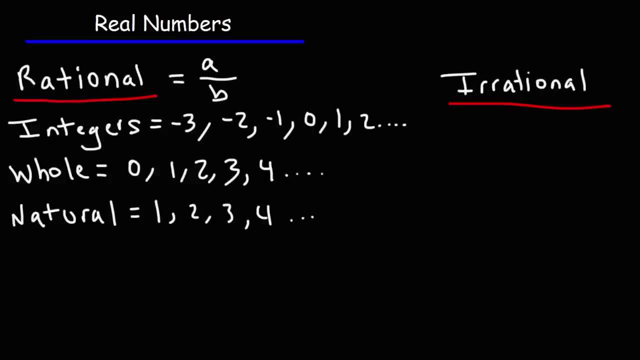 let's talk about the other half of real numbers, that is, irrational numbers. An irrational number cannot be put in a fraction of two integers. So, for instance, the square root of 2, this is equal to 1.414213, and it goes on forever. 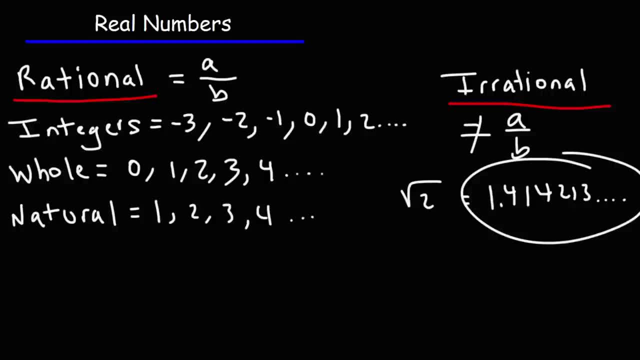 However, you can't write this number in terms of two integers using a fraction Irrational numbers. they tend to be non-repeating decimals and they are non-terminating. They go on forever. You know what? Let's write that down. 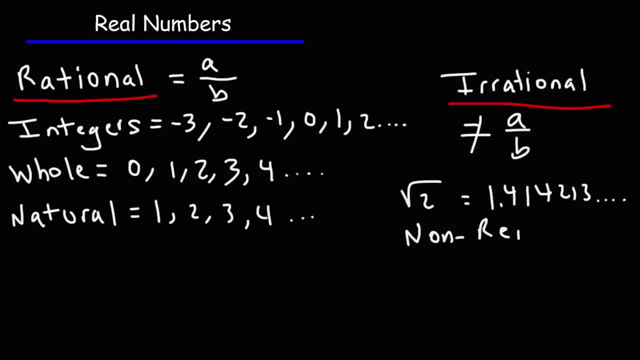 So non-repeating And non-terminating decimals. Another example of this is the number e. If you type in e in your calculator, you'll get 2.7182818, and this just keeps on going. So this is an irrational number. It's non-repeating, non-terminating. 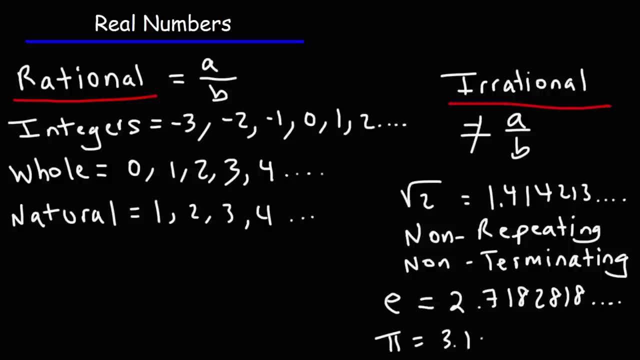 Next we have the number pi. Pi is 3.1415926, and this goes on. That's non-repeating and non-terminating, so that's going to be an irrational number. You can't put pi in terms of. you can't write it as a fraction of two integers. 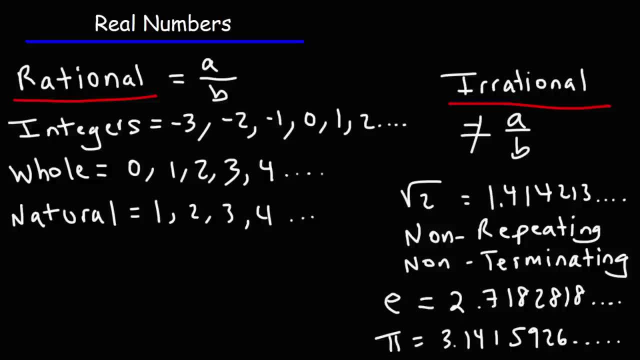 So pi and the square root of 2, those are irrational numbers, But they're still real numbers, though You could plot it on a number line. By the way, for those of you who want to be notified whenever I release specialized content: 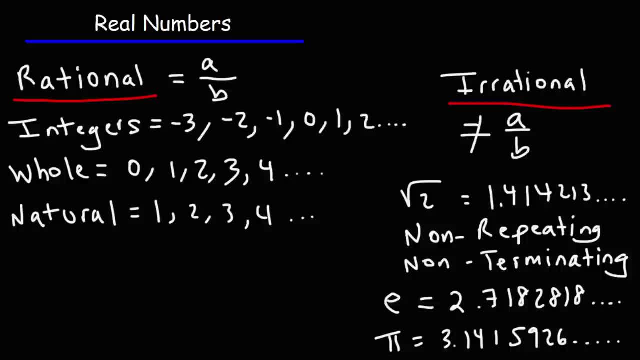 feel free to join my email list. at my website, video-tutornet, I'm going to post a link in the description section below this video, so feel free to take a look at that Now. I do want to mention something regarding e, because it does look like there's a portion that's repeating. 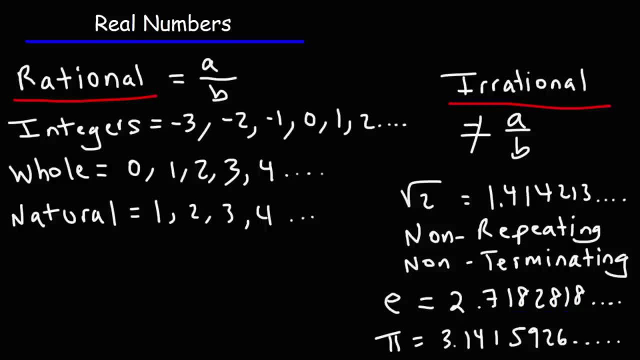 The 1-8,, the 2-8, and the 1-8.. But when you write out this number, you'll see that in the long run it's not repeating: It's 2.7182818.. 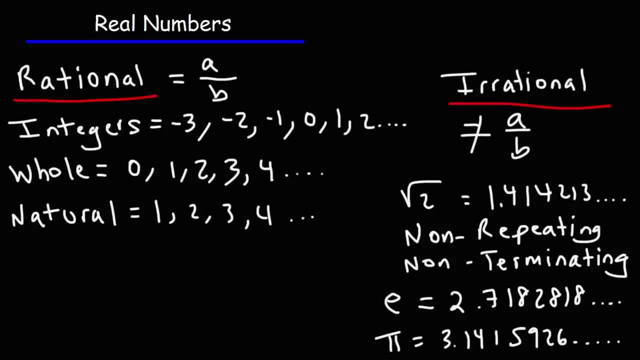 line. by the way, for those of you who want to be notified whenever I release specialized content, feel free to join my email lists. at my website video dash tutor dotnet, I'm gonna post a link in a description section below this video, so feel free to take a look at that now. I 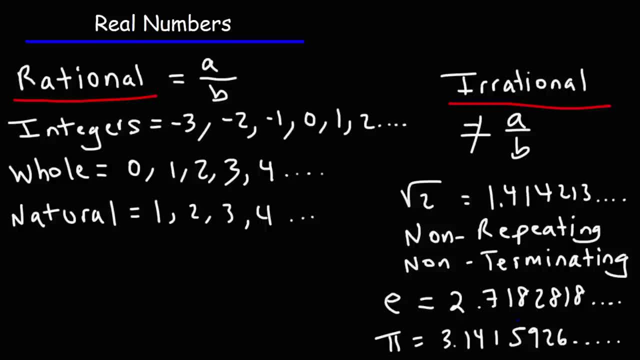 do want to mention something regarding e, because it does look like there's a portion that's repeating the 1: 8, the 2 8 and the 1: 8, but when you write out this number you'll see that in the long run it's not repeating. it's two point seven. 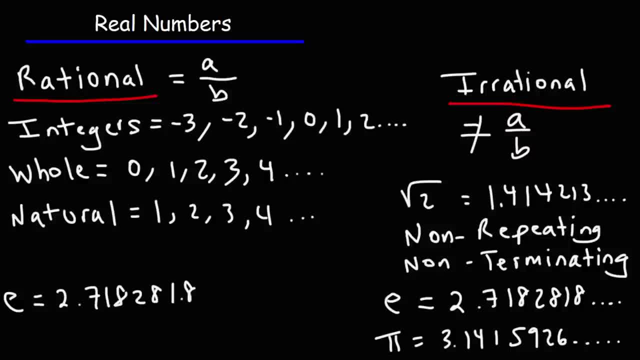 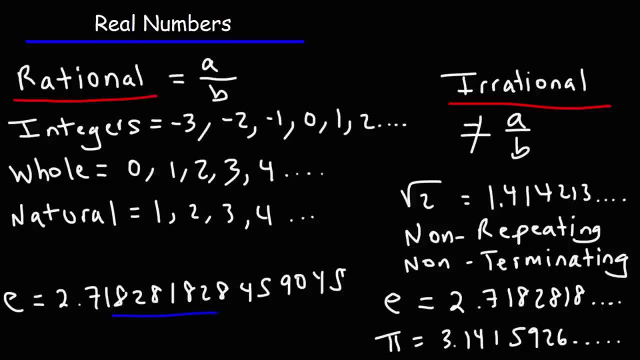 repeating, even though this part appears to be repeating. So E is an irrational number. Now let's go back to rational numbers: 0.375.. This is a non-repeating, but it's a terminating decimal. It doesn't go on forever. 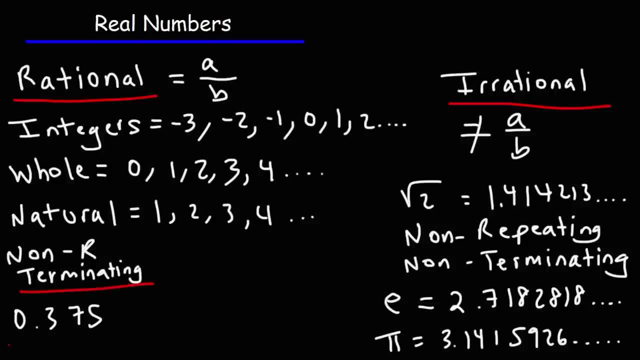 So non-repeating, terminating decimals are rational numbers which are still real numbers. We can put this in the form of a decimal. So we can put this in the form of a decimal As a fraction. this is 375 over 1000.. And of course, you can reduce that fraction. 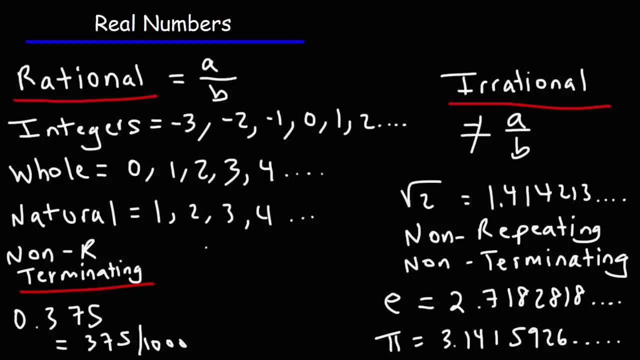 Now the next type of rational number are the ones that have a repeating decimal. It's repeating but non-terminating, So I'll give you an example of that. So 0.2 repeating 0.222222, which we can write that as 0.2 with a bar on top, That's equal to 2 over 9.. 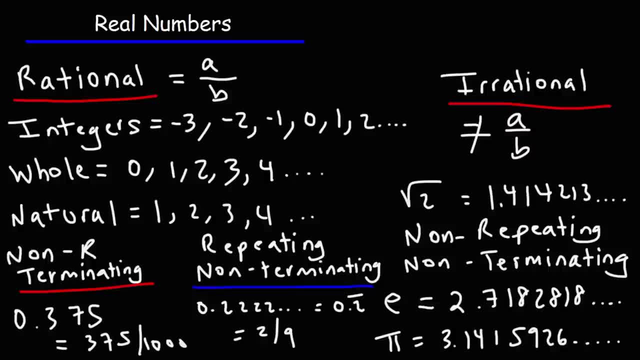 That's a repeating but non-terminating decimal. Another example is 0.44444.. That's 4 over 9.. That's repeating, non-terminating. But note that we can put this as a fraction using two integers. 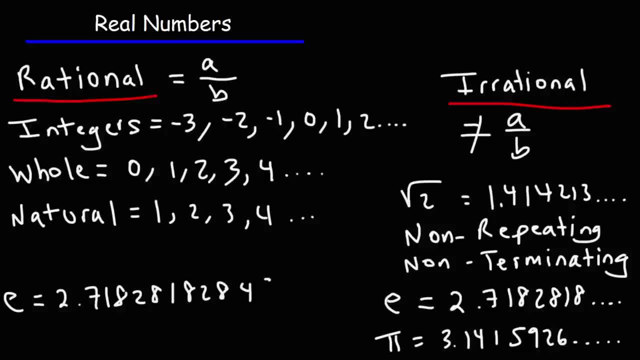 And then there's another 2-8 after that, And then it's 459045.. So ultimately, it's not repeating, even though this part appears to be repeating. So e is an irrational number. Now let's go back to rational numbers. 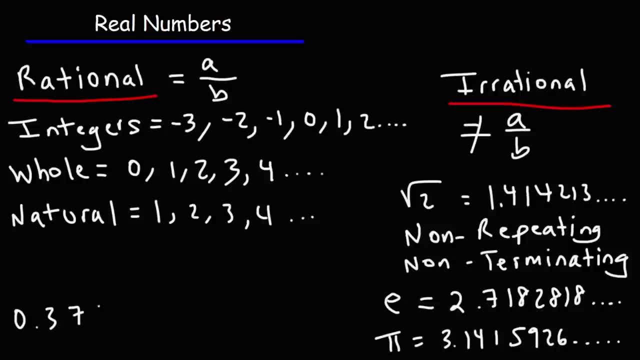 0.375.. This is a non-repeating, but it's a terminating decimal. It doesn't go on forever. So, non-repeating, terminating decimals are rational numbers which are still real numbers. We can put this as a fraction. 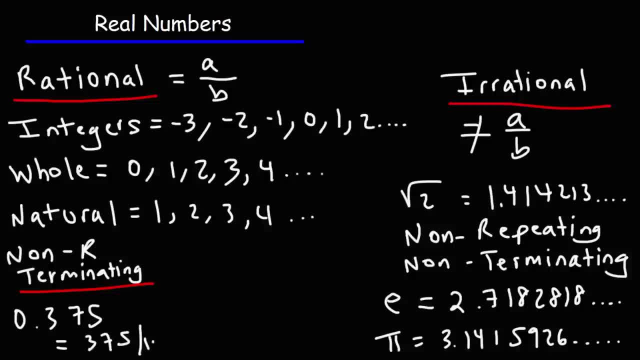 This is 375 over 1000.. And, of course, you can reduce that fraction. Now, the next type of rational number are the ones that have a repeating decimal. It's repeating but non-terminating, So I'll give you an example of that. 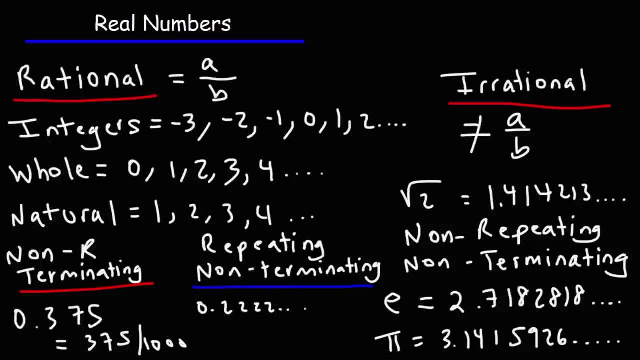 So 0.2 repeating 0.222222, which we can write that as 0.2 with a bar on top, that's equal to 2 over 9.. That's a repeating but non-terminating decimal. Another example is 0.44444. 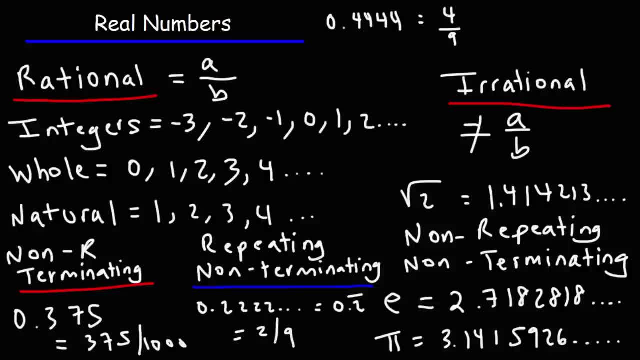 That's 4 over 9.. That's repeating, non-terminating, But note that we can put this as a fraction using two integers. Therefore, these types of decimals are rational numbers, which makes them real numbers. So let me give you another example. 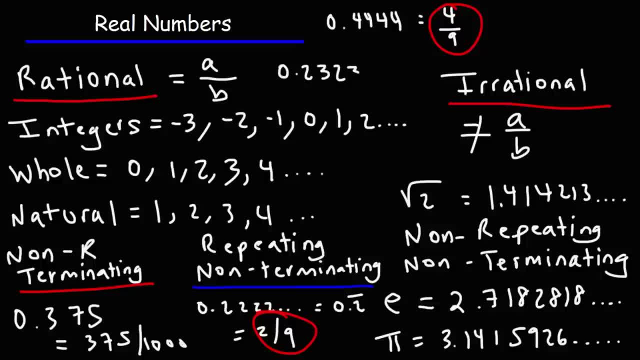 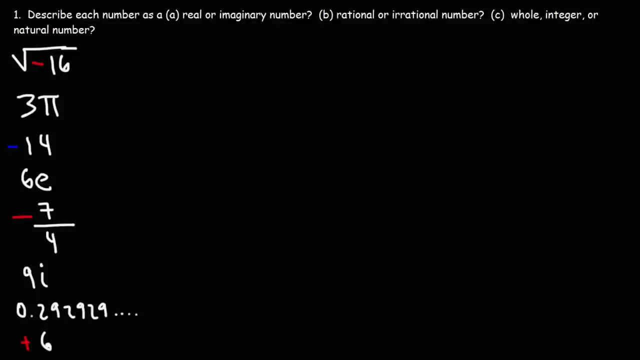 Let's say we have this one, 0.232323.. So this goes on forever. It's repeating but non-terminating. So we can put that as a fraction of two integers. That's 23 over 99,, which makes it a rational number. 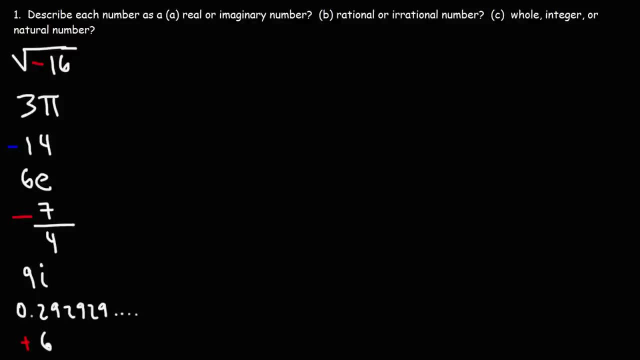 Now let's work on some practice problems. Describe each number as a real or imagined number, rational or irrational, whole, integer or natural number. Feel free to pause the video and work on these problems. By the way, for those of you who need help passing difficult math and science classes. 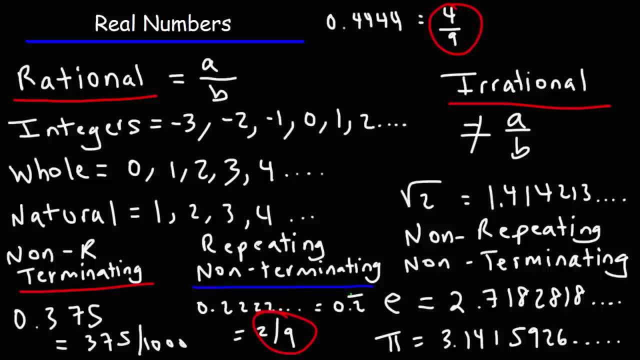 Therefore, these types of decimals are rational numbers, which makes them real numbers. So let me give you another example. Let's say we have this one: 0.232323.. So this goes on forever. It's repeating but non-terminating. 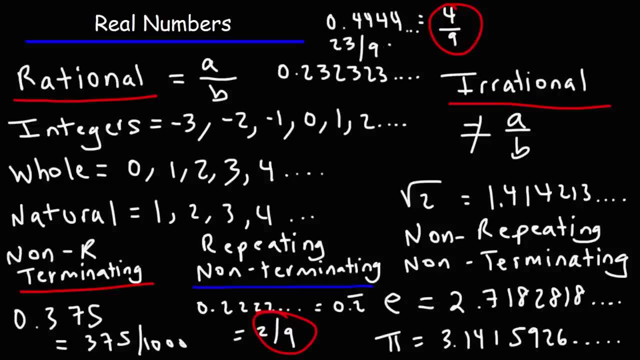 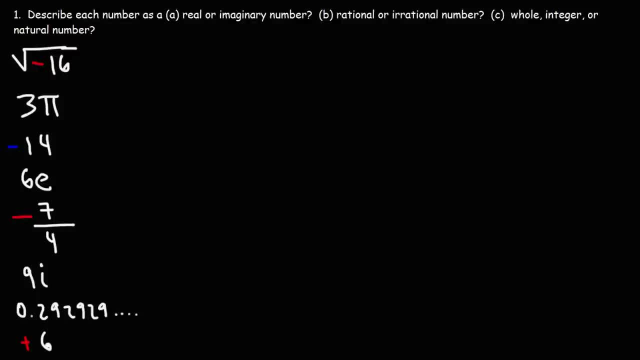 So we can put that as a fraction of two integers, That's 23 over 99, which makes it a rational number. Now let's work on some practice problems. Describe each number as a real or imagined number, rational or irrational, whole, integer or natural number. 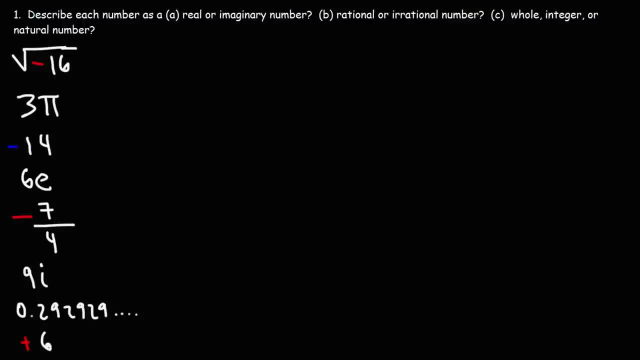 Feel free to pause the video and work on these problems. By the way, for those of you who need help passing difficult math and science classes, I have an e-book on Amazon and it's entitled How to Pass Difficult Math and Science Classes. 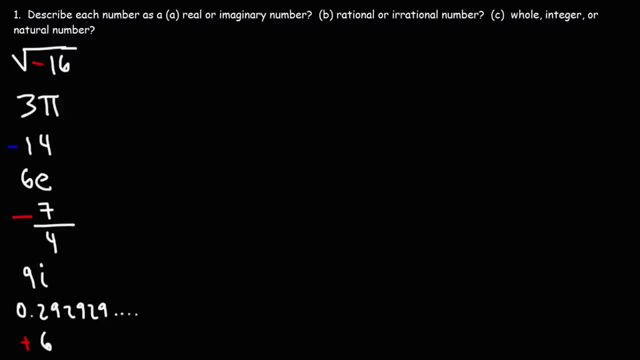 You can look it up on Amazon. You can check the description section below. I'll post a link where you can check it out when you get a chance. So let's go ahead and work on this problem, The square root of negative 16, is it a real number or is it an imagined number? 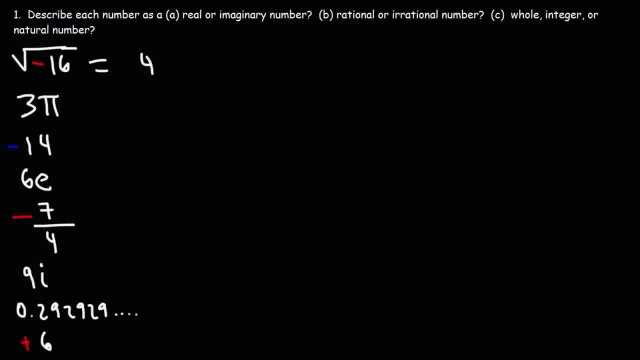 The square root of 16 is 4.. The square root of negative 1 is i. But the way you can simplify it, you can write it like this: This is the square root of 16 times the square root of negative 1.. 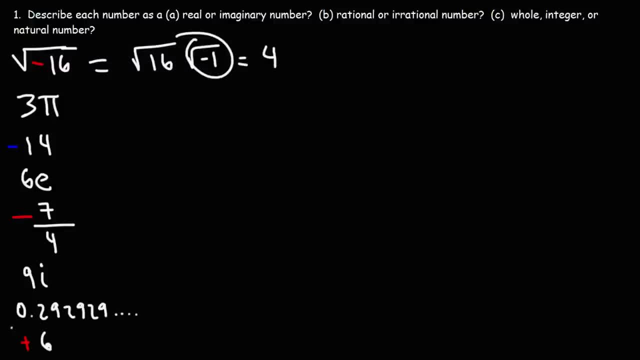 The square root of 16 is 4.. The square root of negative 1 is i. So you get 4i. The fact that there's an i means that it's not a real number. It's going to be an imaginary number. 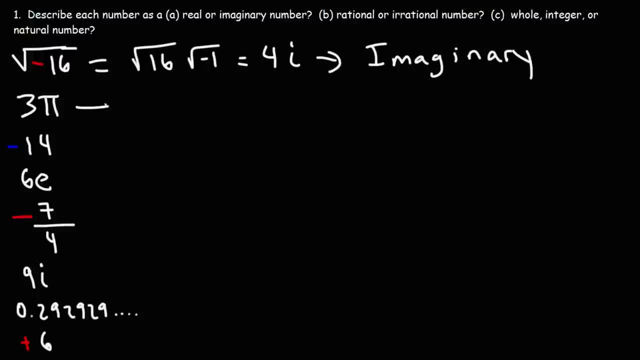 So that's it for the first part of the problem. Now, what about 3pi? Is it real or imaginary? If you don't see, i it's going to be a real number. If it's not imaginary, it's a real number. 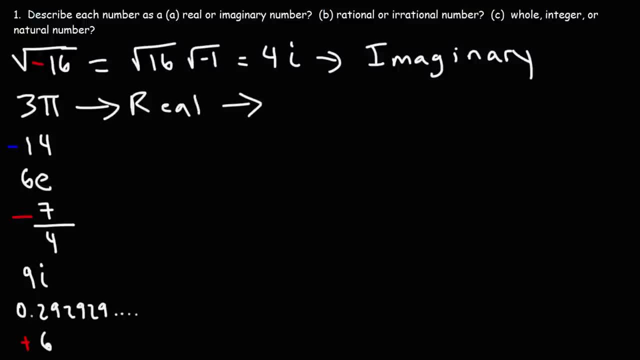 Now we know that pi is a non-repeating, non-terminating decimal. So anytime you see pi, you know it's going to be irrational. And if the number is irrational, that means it's not a whole number, it's not an integer and it's not a natural number. 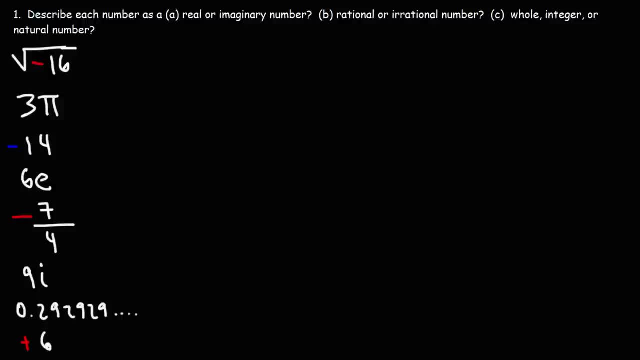 I have an e-book on Amazon and it's entitled How to Pass Difficult Math and Science Classes. You can look it up on Amazon or you can check the description section below. I have a free e-book on Amazon and it's entitled How to Pass Difficult Math and Science Classes. 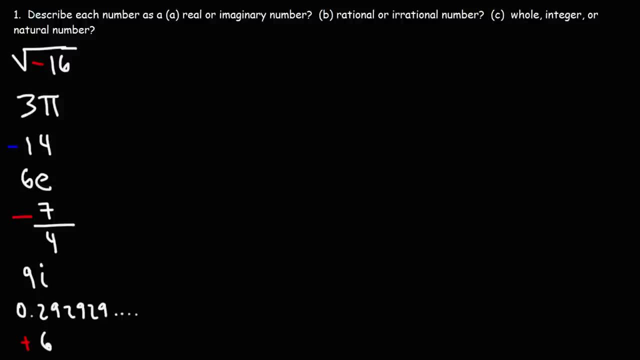 You can look it up on Amazon or you can check the description section below. I'll post a link where you can check it out when you get a chance. So let's go ahead and work on this problem, The square root of negative 16, is it a real number or is it an imagined number? 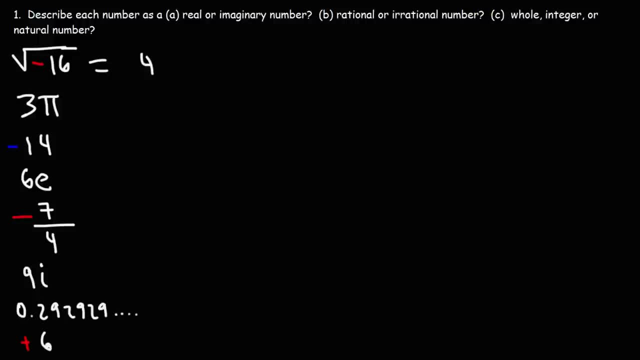 The square root of 16 is 4.. The square root of negative 1 is i. But the way you can simplify it, you can write it like this: This is the square root of 16 times the square root of negative 1.. 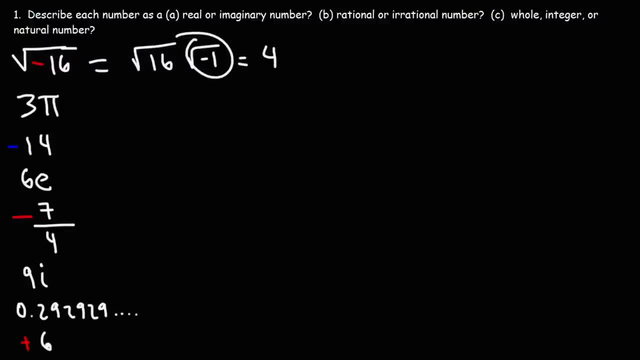 The square root of 16 is 4.. The square root of negative 1 is i. So you get 4i. The fact that there's an i means that it's not a real number. It's going to be an imaginary number. 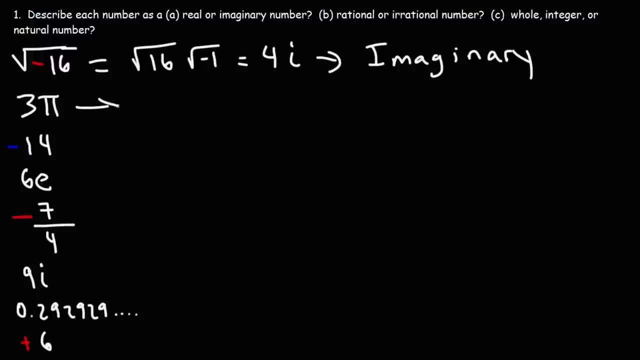 So that's it for the first part of the problem. Now, what about 3pi? Is it real or imaginary? If you don't see, i it's going to be a real number. If it's not imaginary, it's a real number. 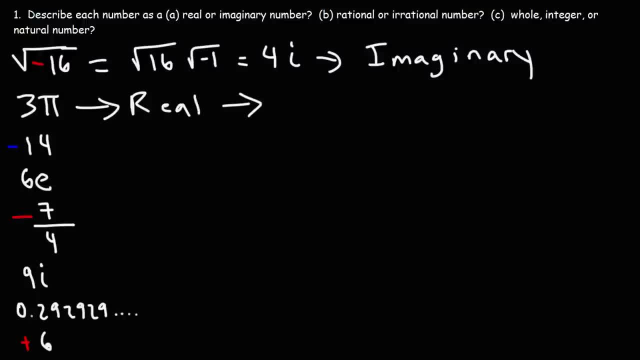 Now we know that pi is a non-repeating, non-terminating decimal. So anytime you see pi, you know it's going to be irrational. And if the number is irrational, that means it's not a whole number, it's not an integer. 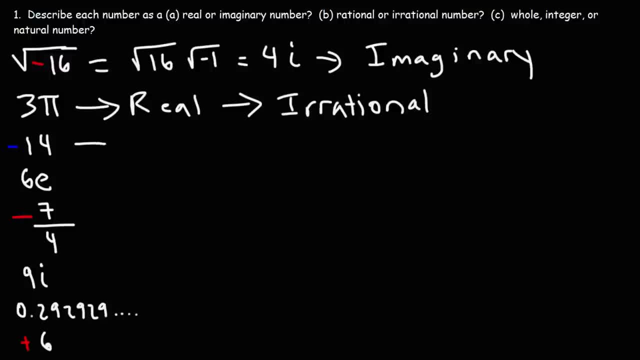 and it's not a natural number. Now, what about negative 14?? There's no i component, so it's not imaginary, It's going to be real. So what about negative 14?? Is it rational or irrational? Negative 14 can be written as a fraction using integers. 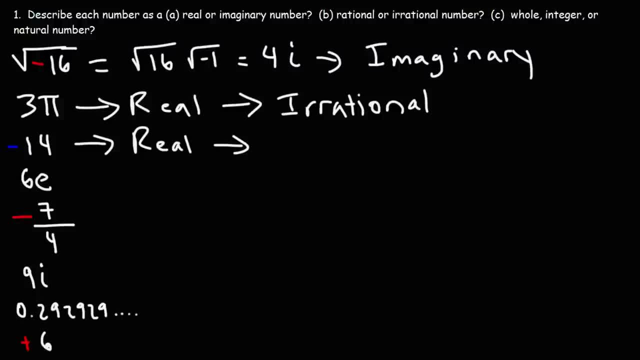 Negative 14 over 1, that's negative 14.. Negative 28 over 2, that's also equivalent to negative 14.. So that makes it rational. Now, negative 14, it's not a whole number, it's not a natural number, but it is an integer. 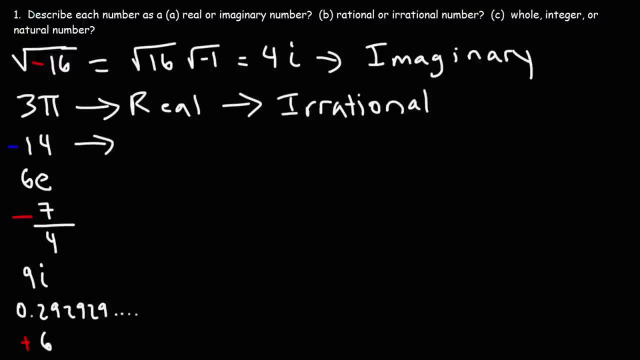 Now what about negative 14?? There's no i component, so it's not imaginary, It's going to be real. Is it rational or irrational? Negative 14 can be written as a fraction using integers. Negative 14 over 1, that's negative 14.. 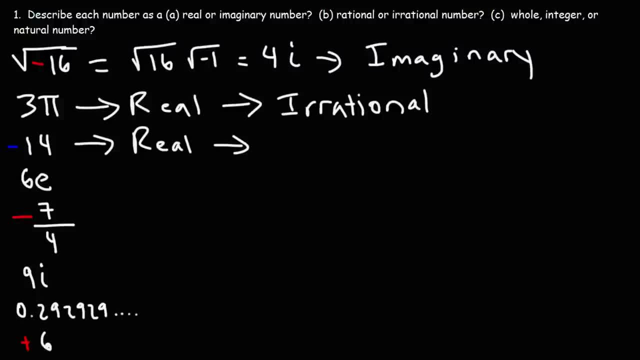 Negative 28 over 2, that's also equivalent to negative 14.. So that makes it rational. Now, negative 14, it's not a whole number, it's not a natural number, but it is an integer. Negative 14 over 1, that's negative 16.. 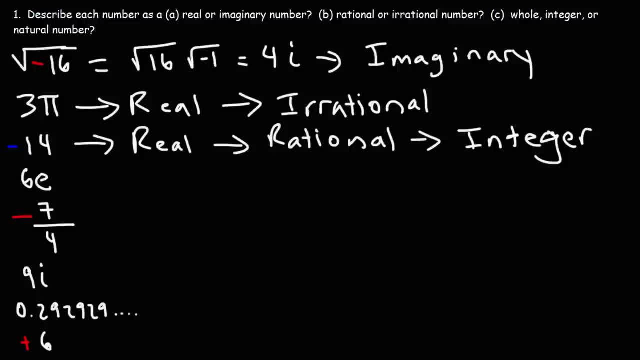 Negative. 4 over 1, that's natural. Negative 1 over 3, that's non-repeating, non-terminating decimal. The number is real. Now, what about 6e? What would you say about that? Well, there's no, i next to it. so it's not imaginary, it's real. 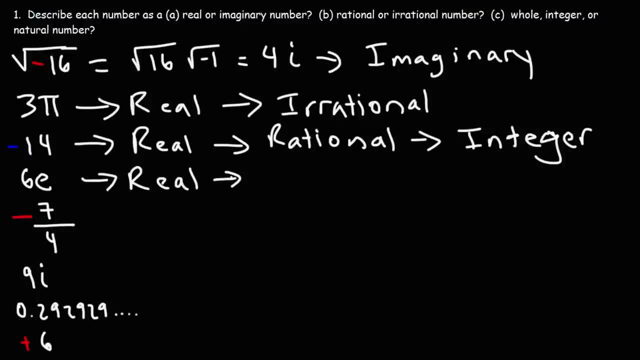 We know the number e is a non-repeating, non-terminating decimal number, so automatically it's going to be irrational. Now what about negative 7? over 4. We can plot that on a number line, so that's going to be a real number, It's. 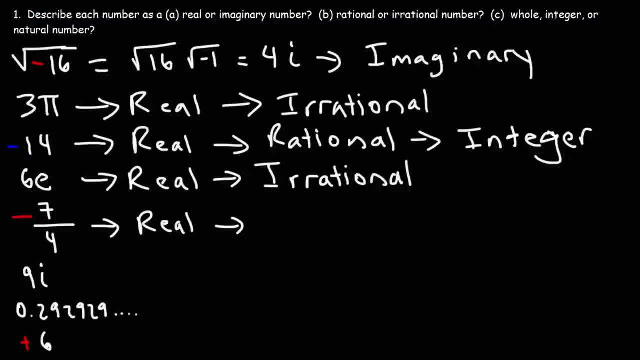 already a fraction using two integers, so it's not irrational. but it's rational Now because it's a fraction. it's not a whole number, it's not an integer, nor is it a natural number. so I'm just going to write fraction 9i. the fact that we have i means it's not real. 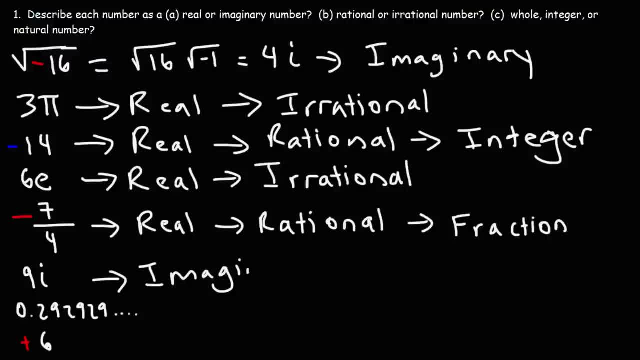 but it's imaginary and that's all we can say about that. 0.29 repeating. so we have a repeating, non-terminating decimal and we can write this as a fraction: This is 29 over 99.. Now you can plug. 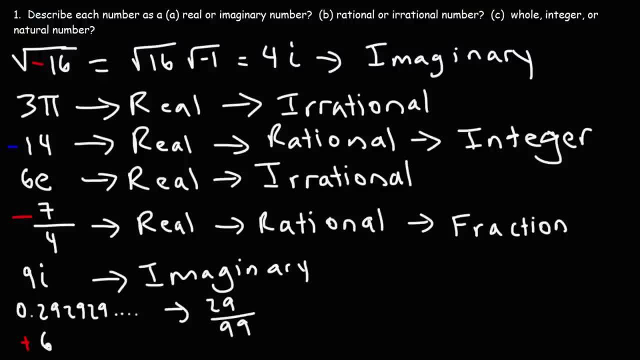 that in your calculator, if you want. So any fraction using integers. that's a real number and it's going to be rational as well. Positive 6,: that is definitely a real number. It's also rational. We can write that as a fraction. 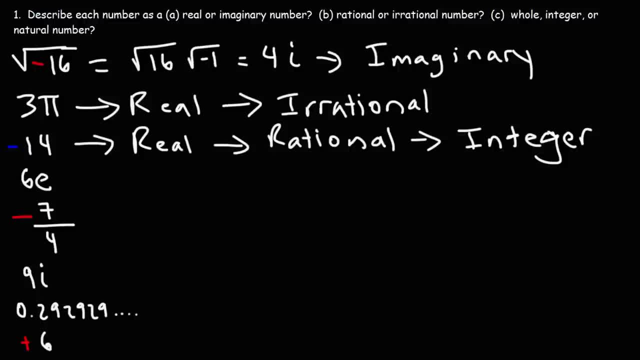 Now what about 6e? What would you say about that? Well, there's no i next to it, so it's not imaginary, it's real. We know the number e is a non-repeating, non-terminating decimal number, so automatically it's going. 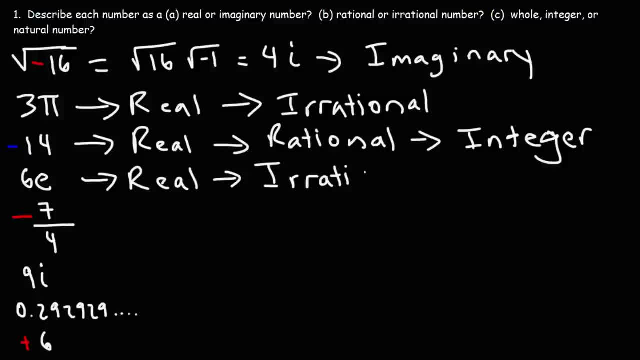 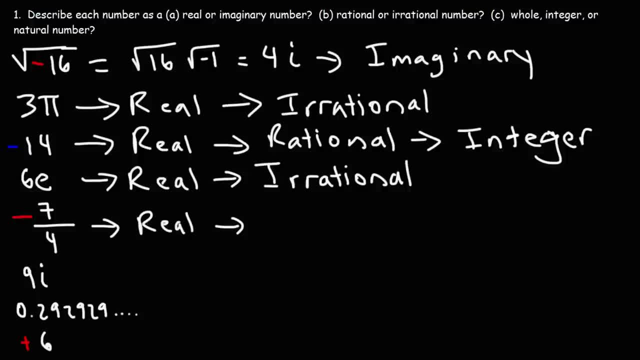 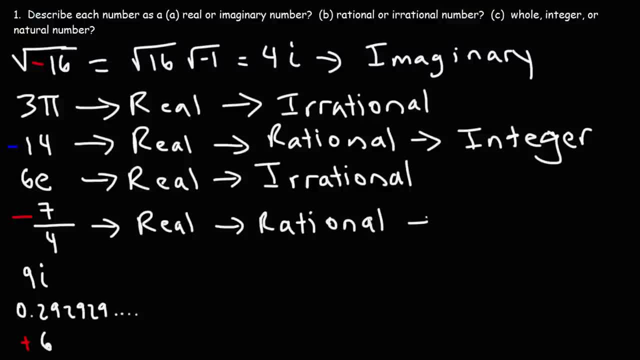 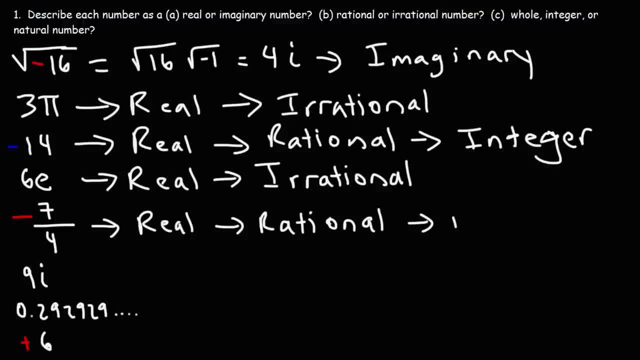 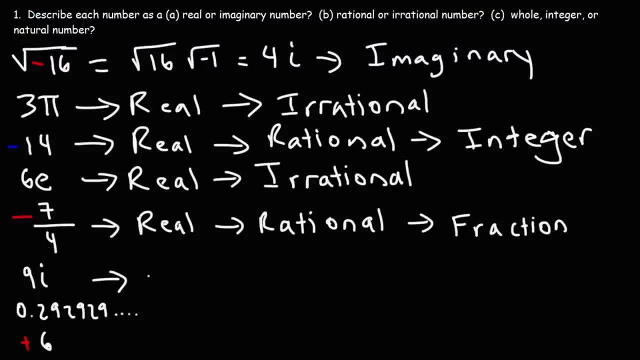 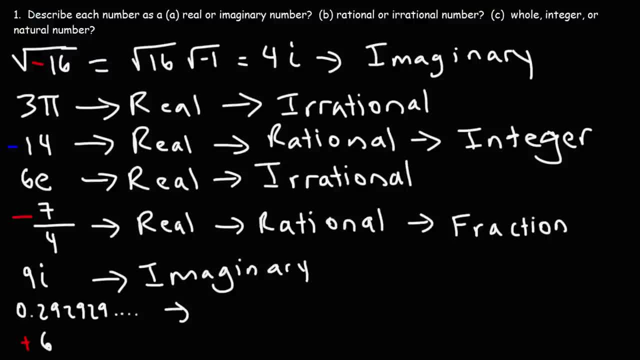 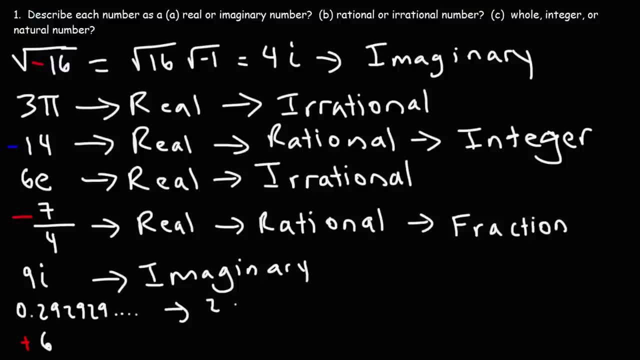 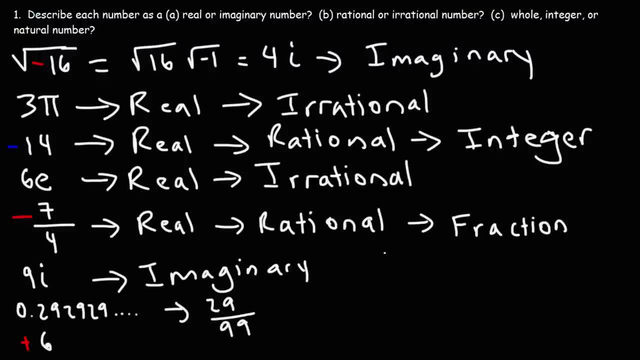 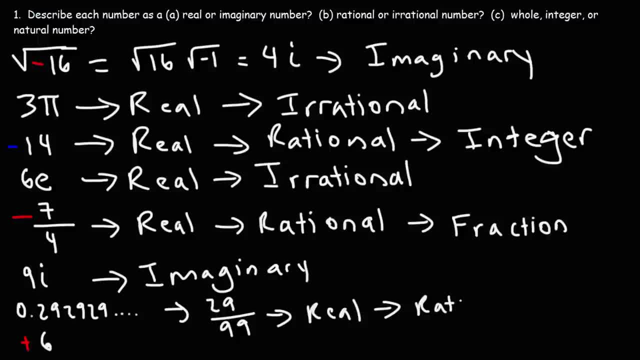 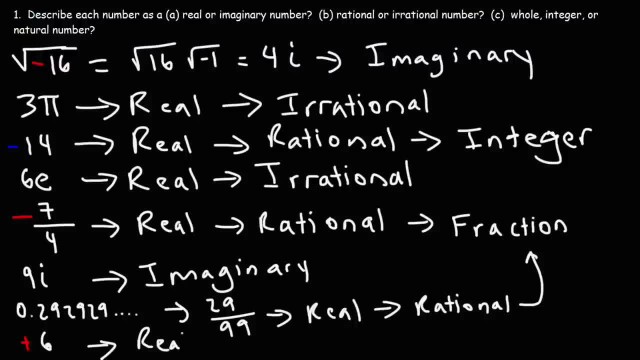 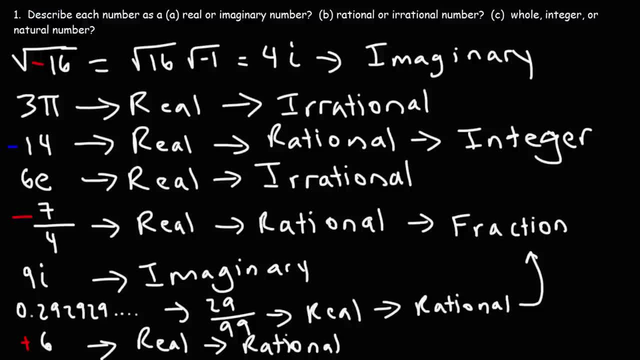 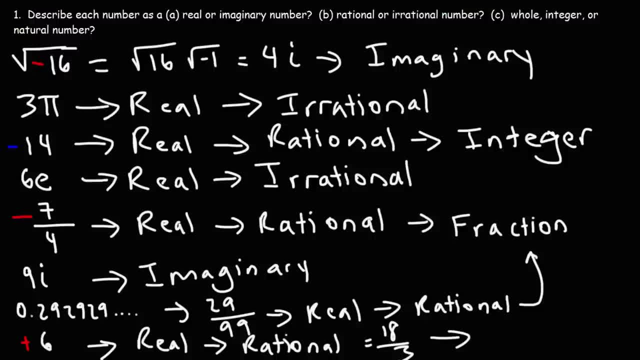 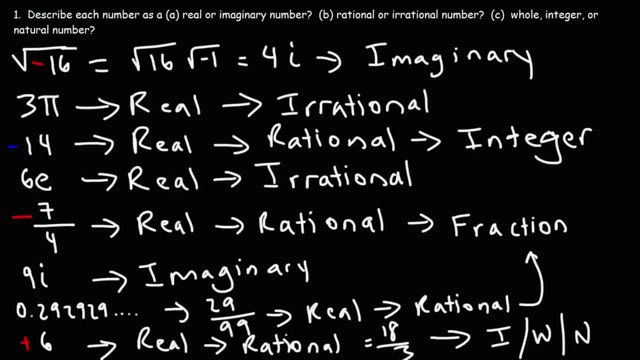 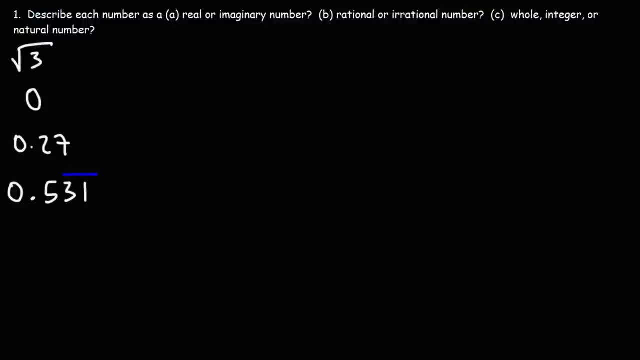 a real number, it's rational, it's an integer, whole number and a natural number at the same time. Go ahead and work on the next four examples. So let's start with the square root of 3.. And what about the square root of 9?? Which one is real and which one is imaginary? Well, none of them. 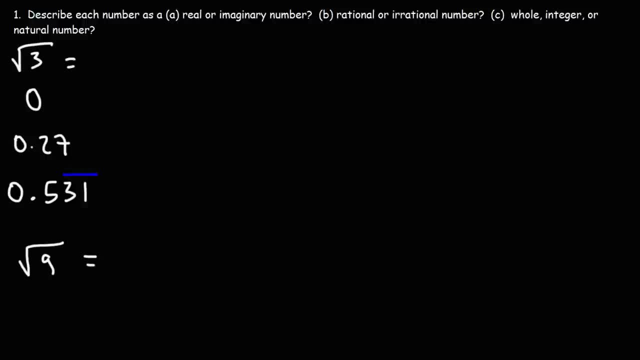 are imaginary. There's no i. We're not dealing with the square root of a negative number, So both of these numbers are real. The square root of 9 simplifies to 3.. So that makes it rational. And because we're dealing with 3, that's an integer. 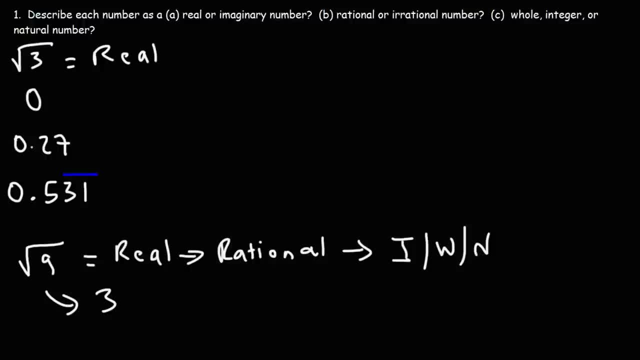 It's a whole number and it's also a natural number. Now, what about the square root of 3?? If you type in the square root of 3, you're going to get 1.73205.. And this keeps on going. 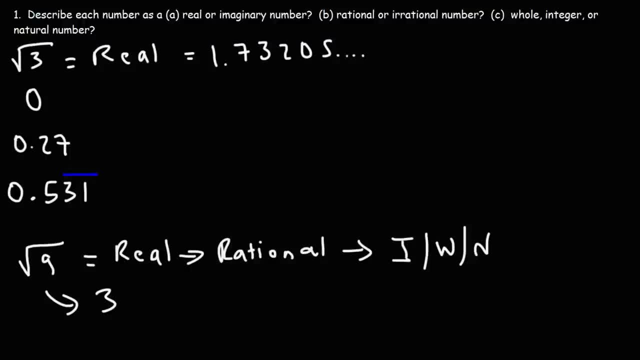 So what we have is a non-repeated, non-terminating decimal. It's a real number, You can plot it on a number line, but you can't write it as a fraction of two integers. So it's not rational, it's irrational. 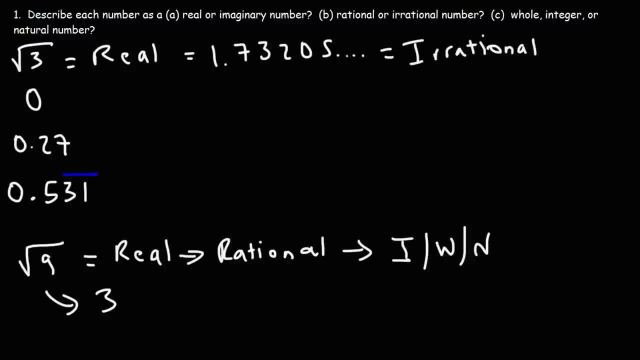 So when dealing with square roots, you need to determine if it simplifies or if it doesn't. If it simplifies to an integer, like the square root of 9, then you know it's going to be real and rational. The square root of negative 25, it simplifies to an integer, but there's an i in. 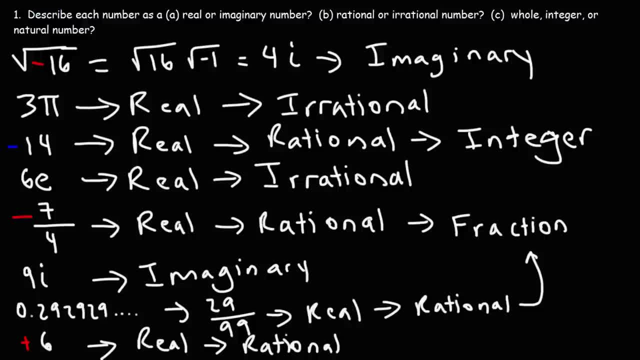 6 over 1,, 12 over 2,, 18 over 3.. Now, positive 6 is an integer, It's also a whole number and it is a natural number. So we could describe it five ways. It's a real number, it's rational, it's an integer, whole number and a. 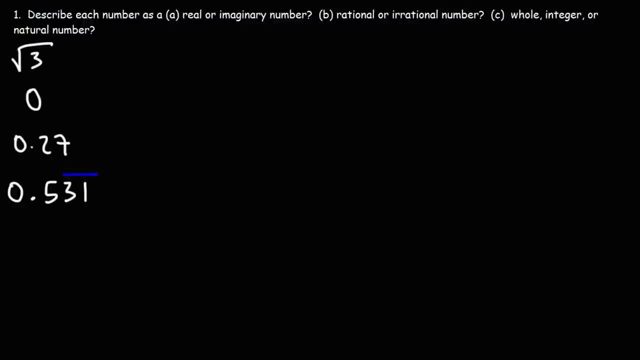 natural number. at the same time, Go ahead and work on the next four examples. So let's start with the square root of 3.. And what about the square root of 9?? Which one is real and which one is imaginary? Well, none of them are. 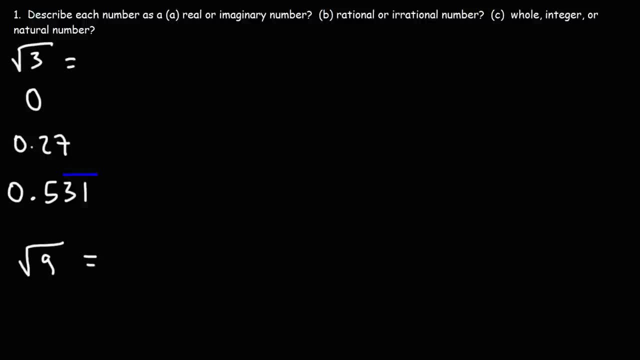 imaginary. There's no i. We're not dealing with the square root of a negative number, So both of these numbers are real. The square root of 9 simplifies to 3.. So that makes it rational. And because we're dealing with 3, that's an integer, It's a whole number and it's also a natural number. 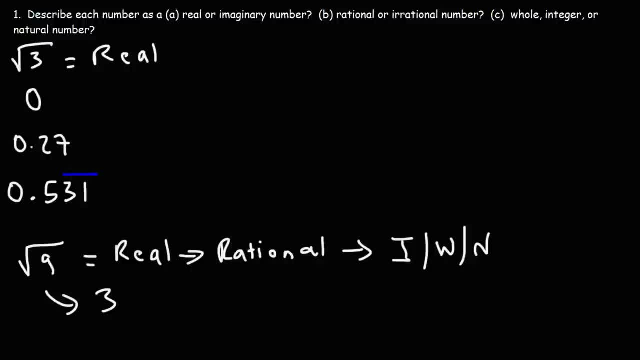 Now what about the square root of 3?? If you type in the square root of 3, you're going to get 1.73205.. And this keeps on going. So what we have is a non-repeated, non-terminating decimal. 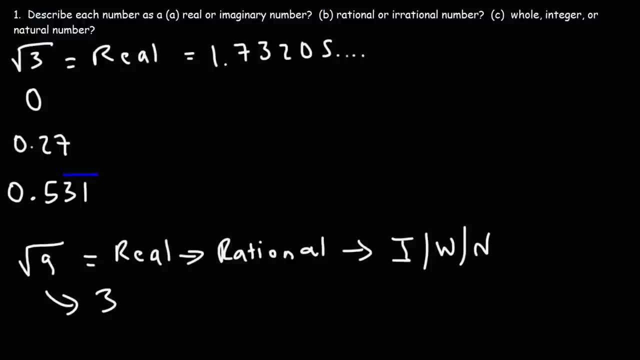 It's a real number, You can plot it on a number line, but you can't write it as a fraction of two integers. So what we have is a non-repeated, non-terminating decimal. It's a real number, You can plot it on a number line, but you can't write it as a fraction of two integers. 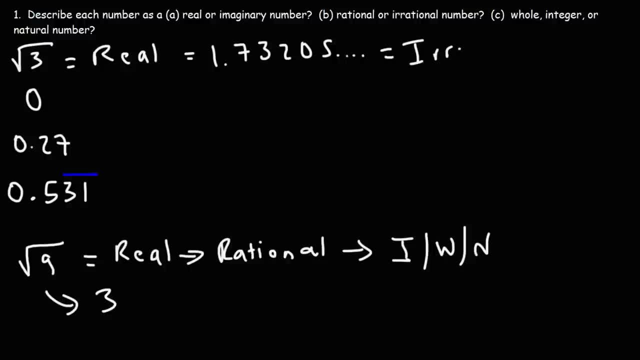 So it's not rational, It's irrational. So when dealing with square roots you need to determine if it simplifies or if it doesn't. If it simplifies to an integer like the square root of 9, then you know it's going to be real and rational. 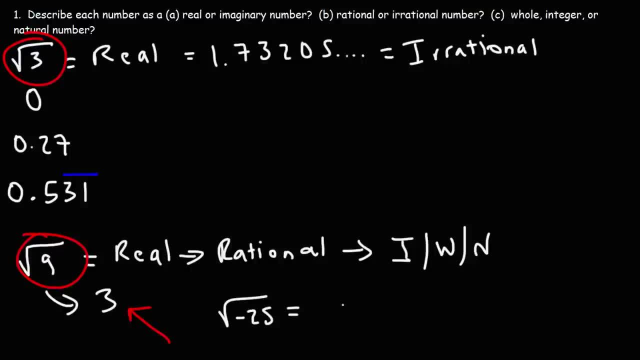 The square root of negative 25, it simplifies to an integer, but there's an i in front of it, so it's not real. So you know that makes it imaginary. Now what about 0?? 0 is a real number. You can plot it on a number line. 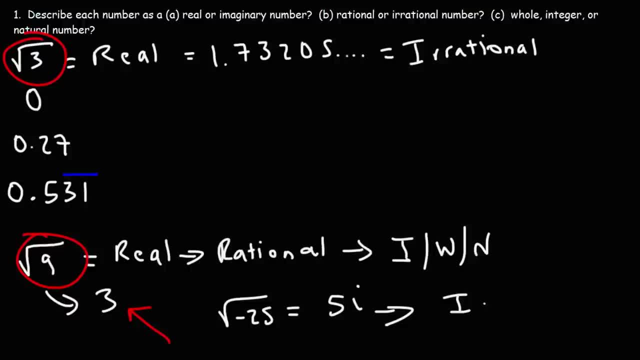 front of it. so it's not real. You know that makes it imaginary. Now what about 0?? 0 is a real number. You can plot it on a number line. It's rational. You can write it as a fraction. 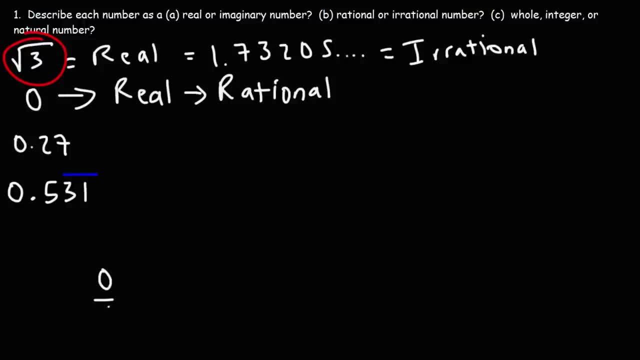 You can write it as a fraction of two integers: 0 over 5, both of these are integers. They equal 0.. 0 over negative 8, they're both integers, They equal 0.. So 0 is rational, It's an integer. 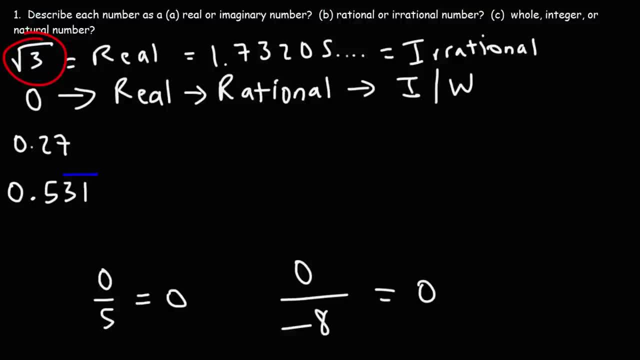 it's a whole number, but it is not a natural number. Now, what about 0.27?? We have a non-repeating terminating decimal. 0.27 can be written as a fraction- 27 over 100, which makes it a rational number. And because it doesn't have an i, next to 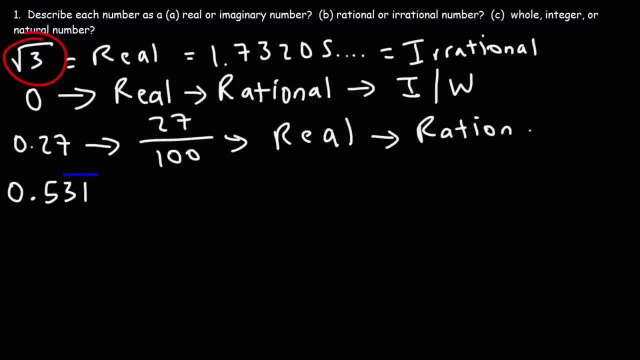 it, it's real. So it's real and it's rational. 0 over 5, both of these are integers. You can plot it on a number line. You can plot it as a fraction, a whole number, integer or natural number. 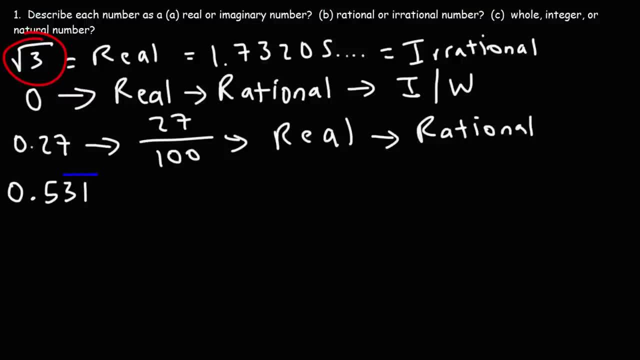 Now, next up, we have 0.531 repeating. The 5 is not repeating, but the 3-1 is. How would you describe this number? Well, we know it's a real number, We can plot it on a number line, But is it rational or irrational? 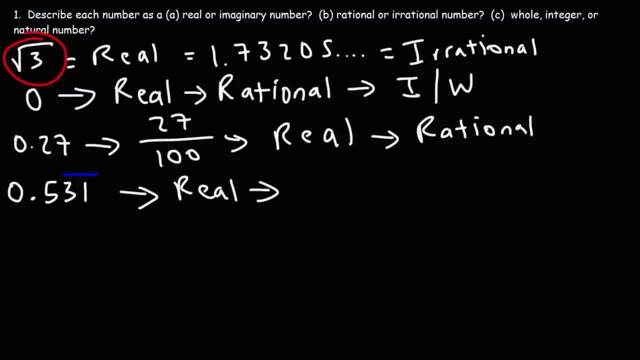 Let's write it out and let's see if we can put it as a fraction of two integers. So this is 0.53.. Well, the 3-1 repeats, so it's going to be 3-1, and then 3-1,, 3-1,, 3-1, and so forth. 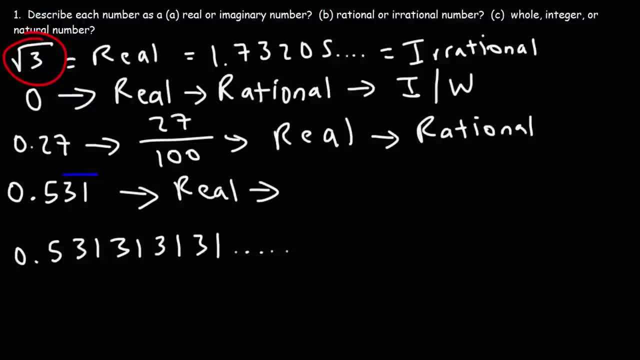 How can we put that into a fraction? Well, we need to identify the repeating element, which appears to be 3-1.. But in actuality, the repeating element is 1-3.. I'm going to add another 3 here. 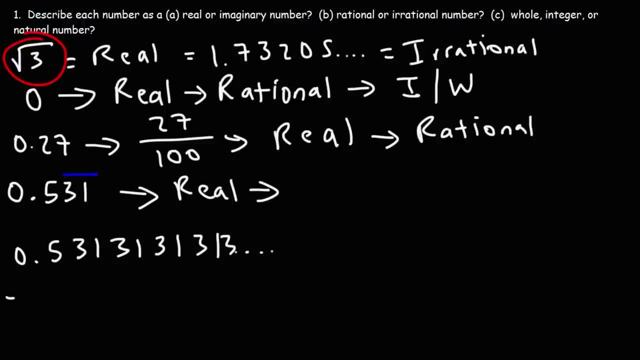 So we're going to subtract this by the repeating element of 0.13.. If you try to subtract it by 0.31, notice that the numbers don't match up. So we're going to add another 3 here. 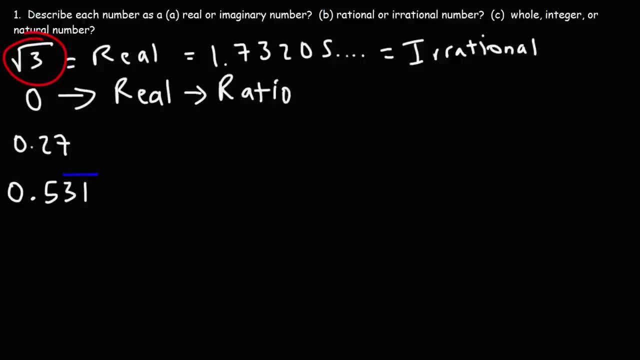 It's rational. You can write it as a fraction. You can write it as a fraction of two integers: 0 over 5, both of these are integers. They equal 0.. 0 over negative 8.. They're both integers. They equal 0.. 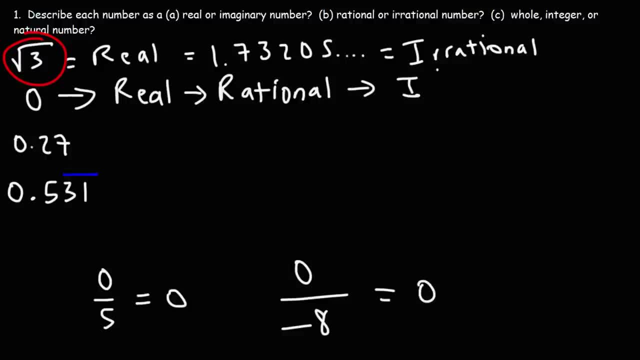 So 0 is rational, It's an integer, It's a whole number, but it is not a natural number. Now, what about 0.27?? We have a non-repeating terminating decimal. 0.27 can be written as a fraction. 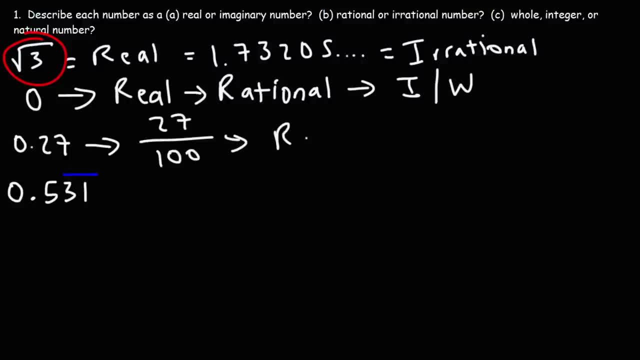 27 over 100, which makes it a rational number. And because it doesn't have an i next to it, it's real, So it's rational. It's real and it's rational, But it's not a whole number, integer or natural number. 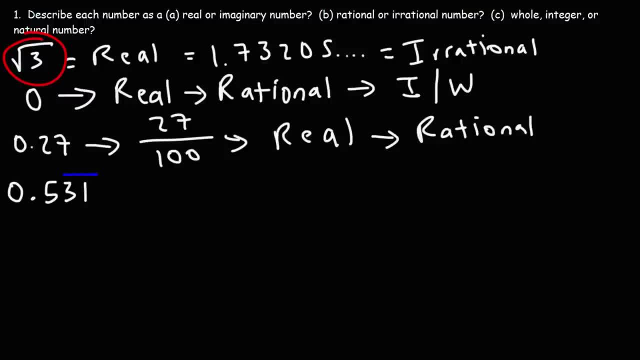 Now, next up, we have 0.531 repeated. The 5 is not repeated, but the 3-1 is. How would you describe this number? Well, we know it's a real number. We can plot it on a number line. 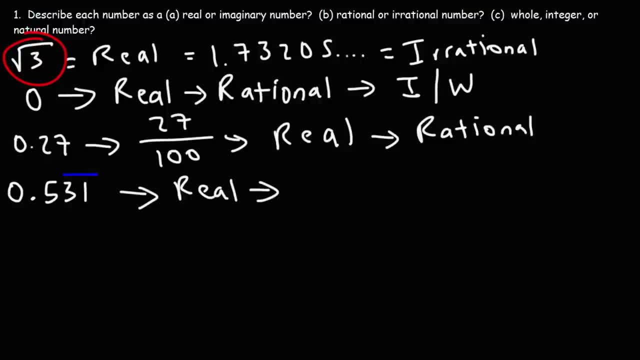 But is it rational or irrational? Let's write it out And let's see if we can put it as a fraction of two integers. So this is 0.53.. Well, the 3-1 repeats, so it's going to be 3-1, and then 3-1,, 3-1,, 3-1, and so forth. 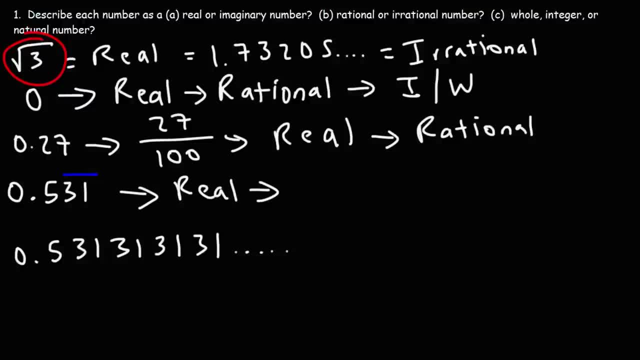 How can we put that into a fraction? Well, we need to identify the repeating element, which appears to be 3-1.. But in actuality, the repeating element is 1-3.. I'm going to add another 3 here. 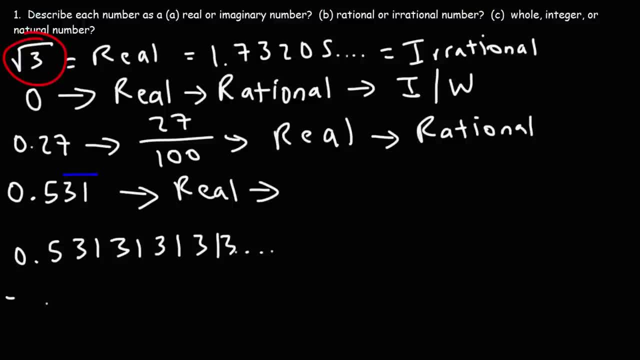 So we're going to subtract this by the repeating element of 0.13.. If you try to subtract it by 0.31, notice that the numbers don't match up. This 1 does not correspond to this 3, and this 3 does not correspond to the 1.. 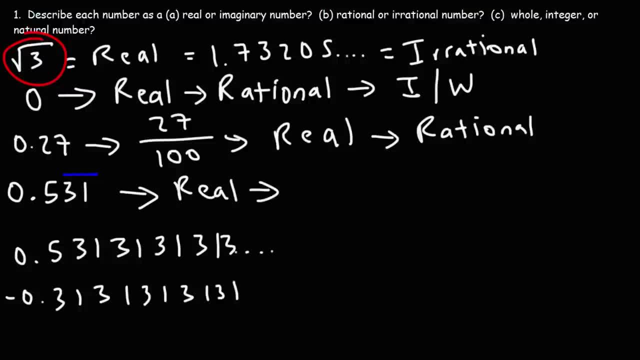 Now let's try that again. We're going to add another 3 here does not correspond to this tree and this tree does not correspond to the one. so therefore it's not 3: 1, but it's actually 1: 3 if we subtract the first. 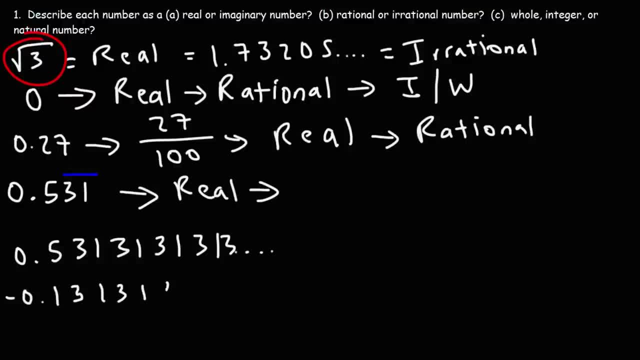 number by point 1, 3 repeating. note that the numbers match up, so this part right here cancels with this part. so we have point 53 minus point 13, which is point 4. so 0.4 is the non-repeating part of this number. so what does that mean? 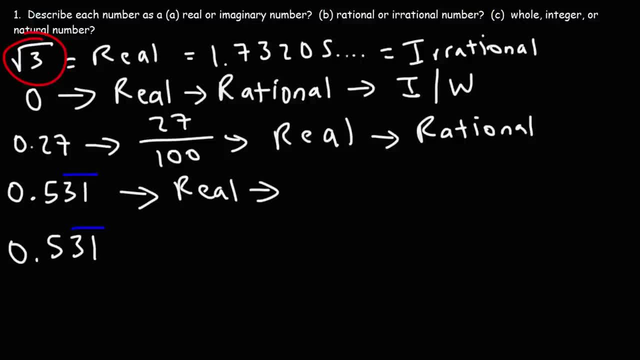 0.5, 3, 1, repeating, which is. this number can be written as 0.4 plus 0.13, 1313, so forth, or 0.13 1313, so forth, or 0.13 1313, so forth, or point 1, 3, repeating, when you add these two. 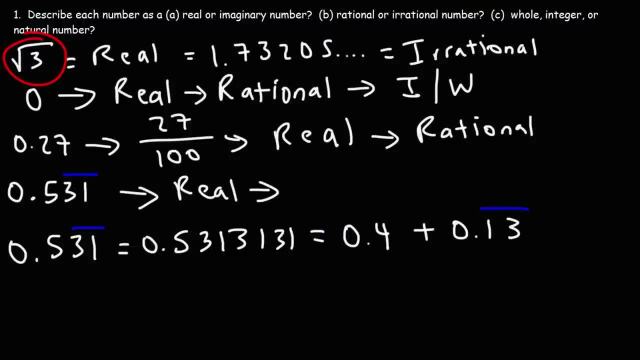 point 1- 3. repeating when you add these two: point 1- 3. repeating when you add these two numbers. you get this number now 0.4 numbers. you get this number now 0.4 numbers. you get this number now 0.4. we can write that as a fraction, that's 4. 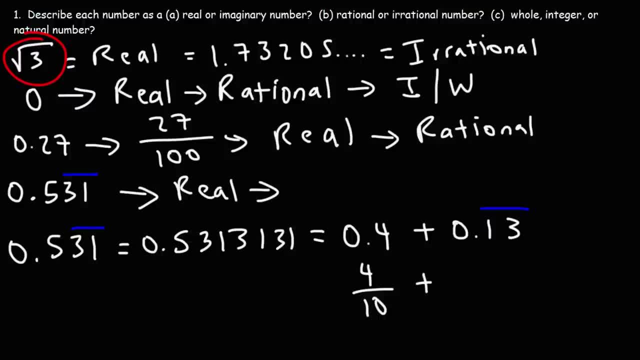 we can write that as a fraction, that's 4. we can write that as a fraction, that's 4 over 10. point 13, repeating. we can write over 10, point 13 repeating. we can write over 10: point 13 repeating. we can write that as a fraction, that's 13 over 99 now. 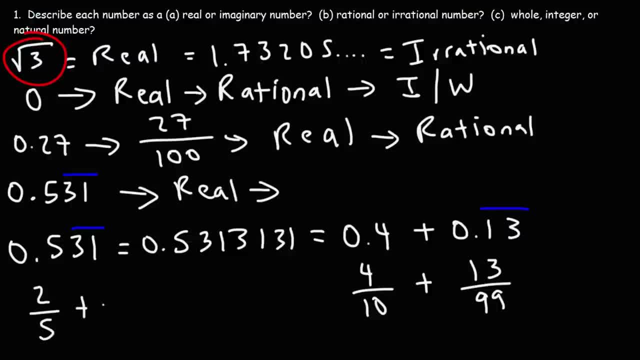 that as a fraction, that's 13 over 99. now that as a fraction, that's 13 over 99, now 4 over 10, we can write that as 2 over 5. 4 over 10. we can write that as 2 over 5. 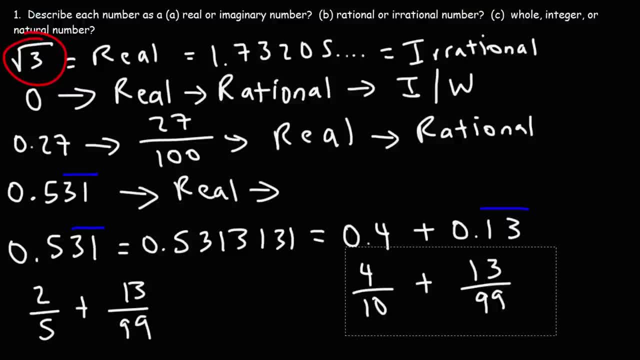 4 over 10. we can write that as 2 over 5. so to combine this into a, so to combine this into a, so to combine this into a single fraction, we need to get common single fraction. we need to get common single fraction. we need to get common denominators. I'm going to multiply the. 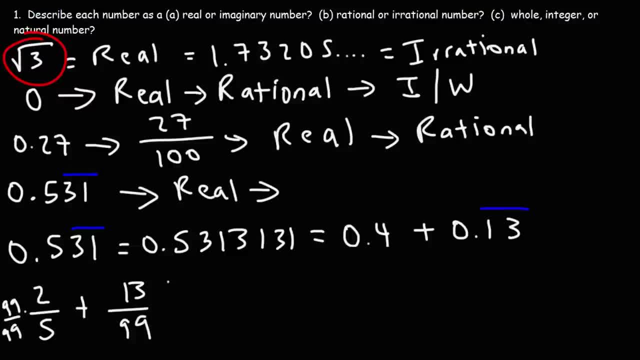 denominators. I'm going to multiply the denominators. I'm going to multiply the first fraction by 99 over 99 and the first fraction by 99 over 99 and the first fraction by 99 over 99 and the second fraction by 5 over 5 2 times 99. 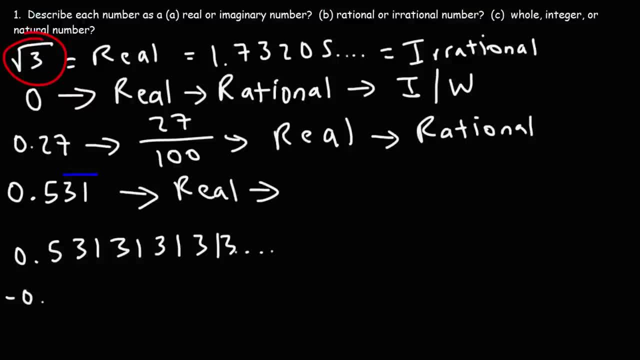 So therefore it's not 3-1, but it's actually 1-3.. If we subtract the first number by 0.13, repeating, note that the numbers match up. So this part right here cancels with this part. 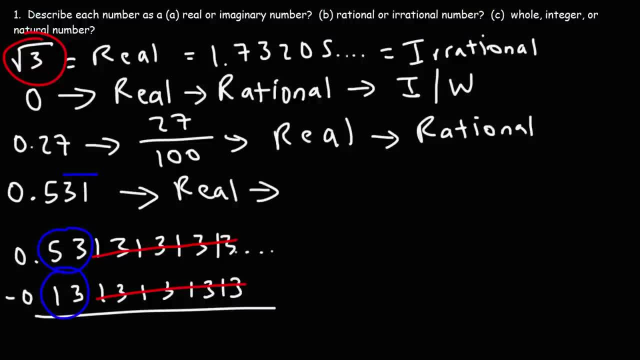 So we have 0.53. And this part here cancels with this part. So 0.53 minus 0.13, which is 0.4.. So 0.4 is the non-repeating part of this number. 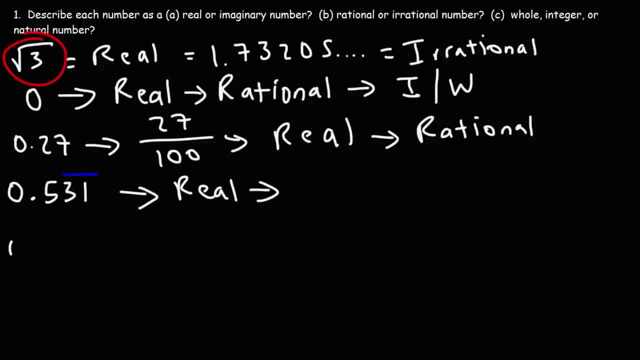 So what does that mean? 0.531, repeating, which is. this number can be written as 0.4 plus 0.123.. 0.13, 1.3, 1.3, so forth, or 0.13 repeating. 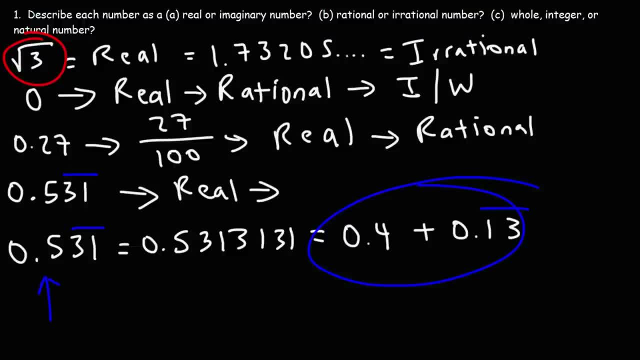 When you add these two numbers, you get this number Now 0.4,. we can write that as a fraction, That's 4 over 10.. 0.13 repeating: we can write that as a fraction, That's 13 over 99.. 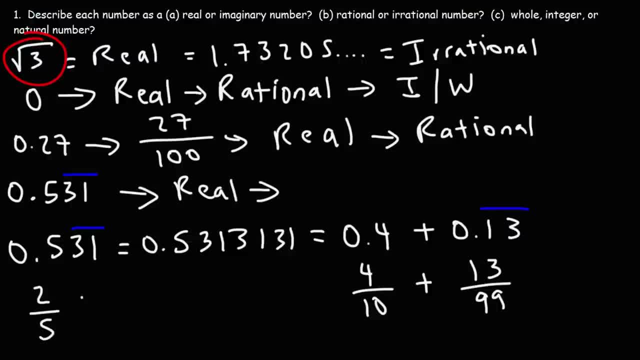 Now 4 over 10, we can write that as 2 over 5.. So to combine this into a single fraction, we need to get common denominators. I'm going to multiply the first fraction by 99 over 99,. 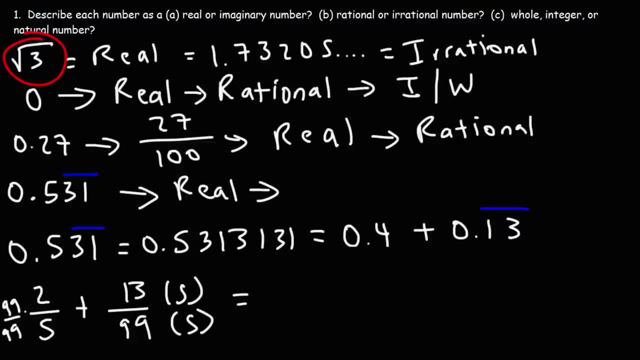 and the second fraction by 5 over 5.. 2 times 99 is 198.. 5 times 99 is 495.. And then 13 times 5 is 65.. 198 plus 65 is 263.. So you can type this in your calculator. 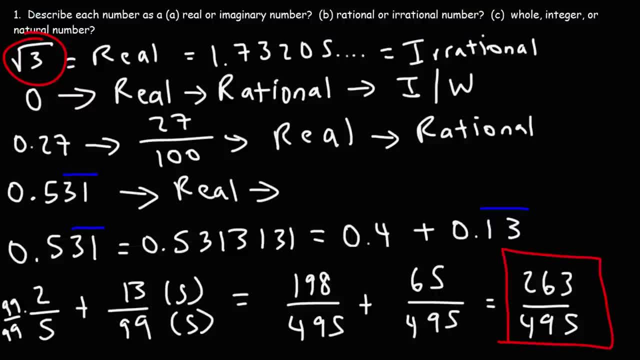 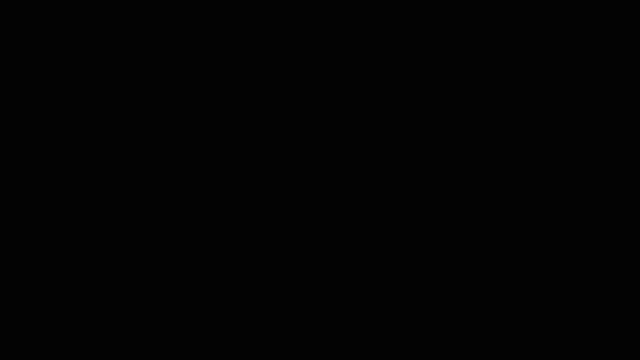 Type in: 263 divided by 495.. And you should get 0.531. repeating, You should get this number. So the fact that we can put it as a fraction of two integers means that it's a rational number. Now let's consider some examples with cube roots. 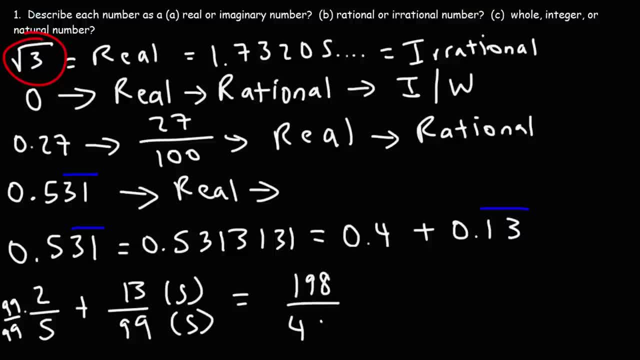 second fraction by 5 over 5, 2 times 99. second fraction by 5 over 5, 2 times 99 is 198. 5 times 99 is 495, and then 13 is 198. 5 times 99 is 495 and then 13. 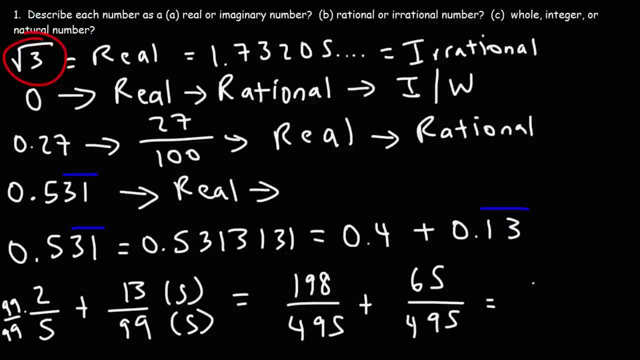 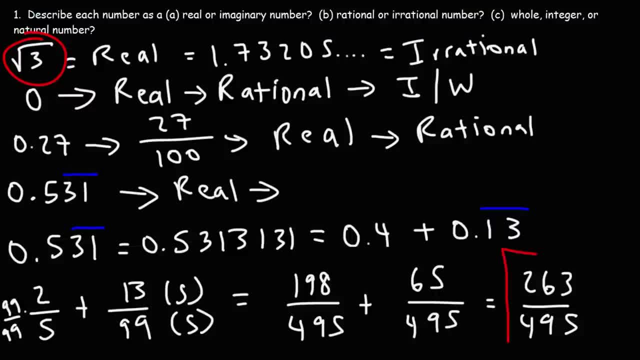 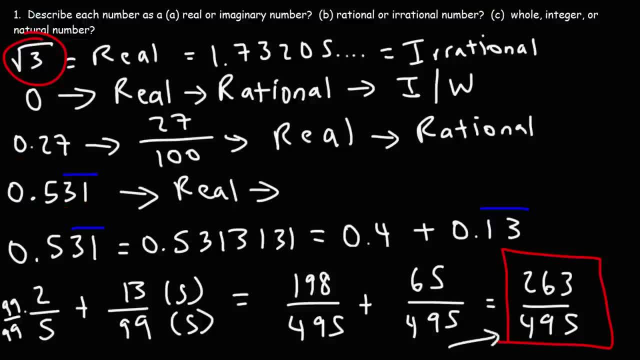 5 3 1. repeating you should get this: 5 3, 1. repeating you should get this number. so the fact that we can put it as number, so the fact that we can put it as number, so the fact that we can put it as a fraction of two integers, means that 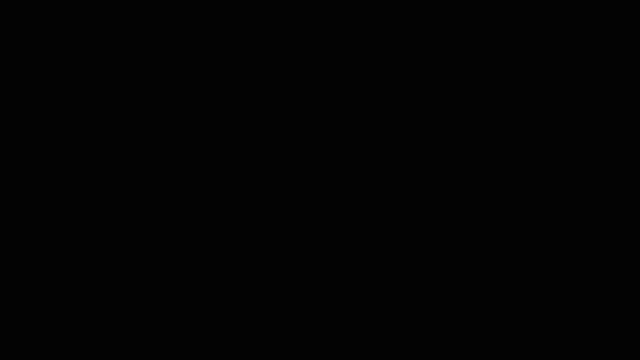 a fraction of two integers means that a fraction of two integers means that it's a rational number. now let's, it's a rational number. now let's, it's a rational number. now. let's consider some examples with cube roots. consider some examples with cube roots. consider some examples with cube roots, given that we've considered a lot of. 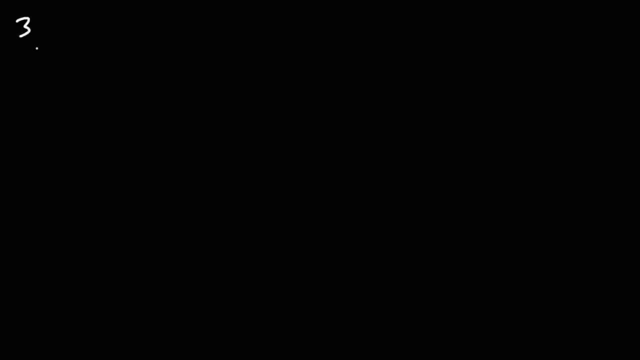 given that we've considered a lot of, given that we've considered a lot of examples with square roots, so let's examples with square roots. so let's examples with square roots. so let's start with the cube root of 8 and then start with the cube root of 8 and then. 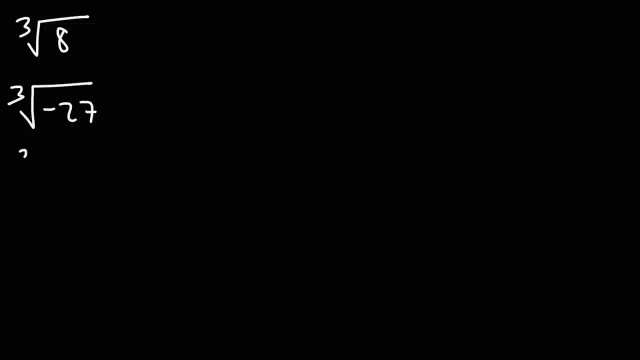 start with the cube root of 8 and then we'll have the cube root of negative 27, we'll have the cube root of negative 27, we'll have the cube root of negative 27 and the cube root of 10 and then the. and the cube root of 10 and then the. 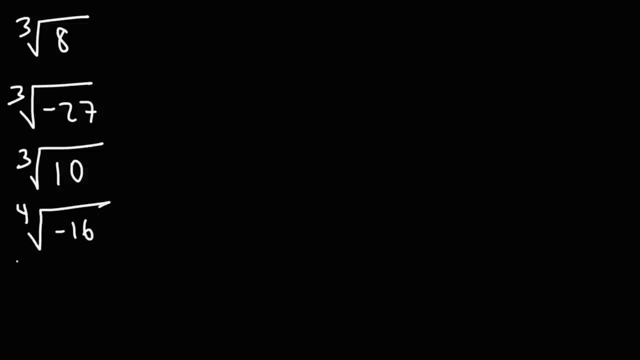 and the cube root of 10, and then the fourth root of negative 16, the fourth fourth root of negative 16, the fourth fourth root of negative 16, the fourth root of 81 and the fourth root of 20. so, root of 81 and the fourth root of 20, so 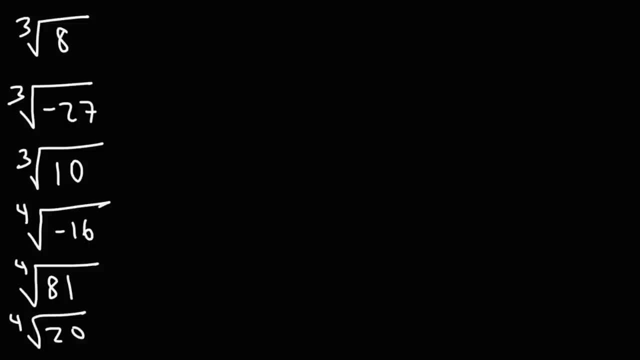 root of 81 and the fourth root of 20, so the cube root of 8, the cube root of 8, the cube root of 8. how would you describe that well first? how would you describe that well first? how would you describe that well first? see if you can simplify the cube root of. 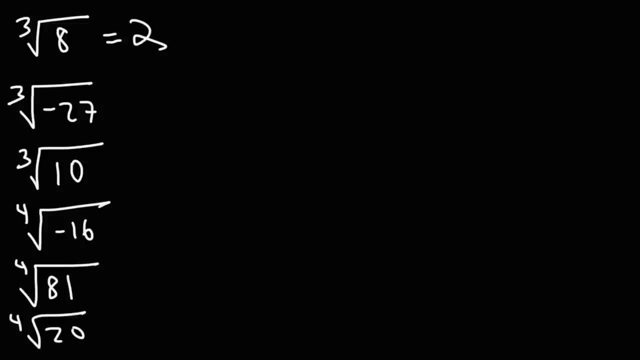 see if you can simplify the cube root of. see if you can simplify the cube root of: 8 is 2 because 2 times 2 times 2, 3 times. 8 is 2 because 2 times 2 times 2, 3 times. 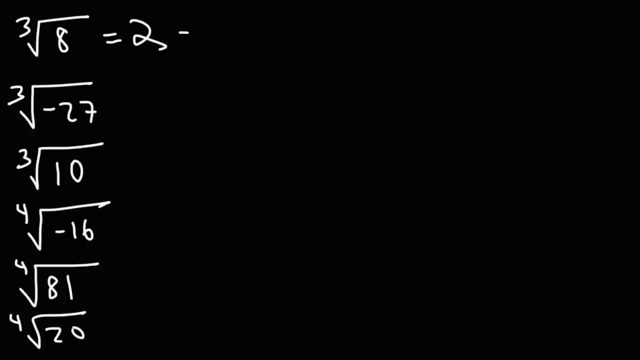 8 is 2, because 2 times 2 times 2, 3 times is 8. so we could simplify that into: an is 8. so we could simplify that into an is 8. so we could simplify that into an integer which makes it real it's. 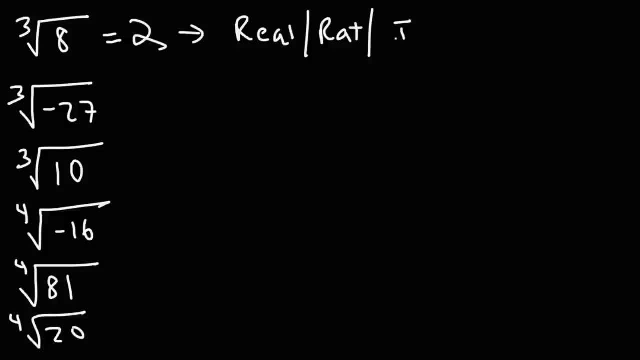 integer which makes it real. it's integer which makes it real. it's rational and it's an integer. it's also a rational and it's an integer. it's also a rational and it's an integer. it's also a whole number and a natural number. now, 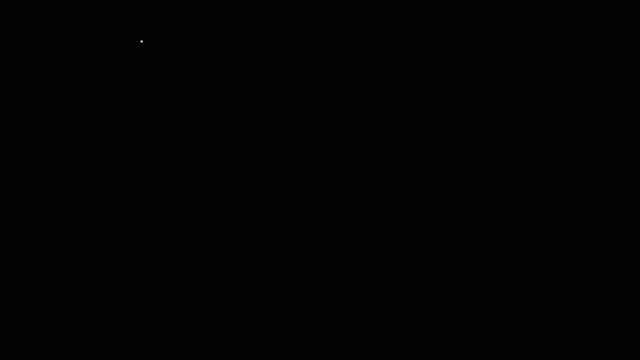 Given that we've considered a lot of examples with square roots. So let's start with the cube root of 8. And then we'll have the cube root of negative 27. And the cube root of 10. And then the fourth root of negative 16.. 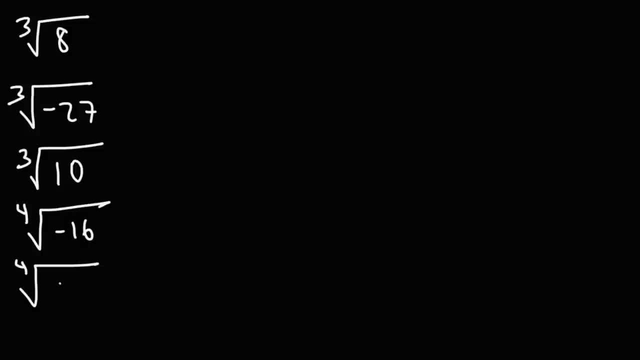 The fourth root of 81. And the fourth root of 20. So the cube root of 8 is negative 27.. So the cube root of 8. How would you describe that? Well, first see if you can simplify it. 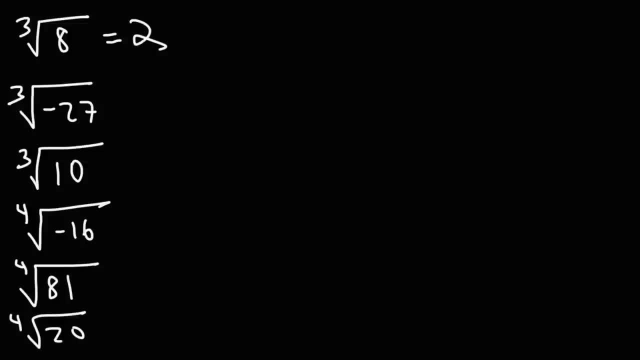 The cube root of 8 is 2.. Because 2 times 2 times 2, 3 times is 8.. So we could simplify that into an integer Which makes it real, It's rational And it's an integer. 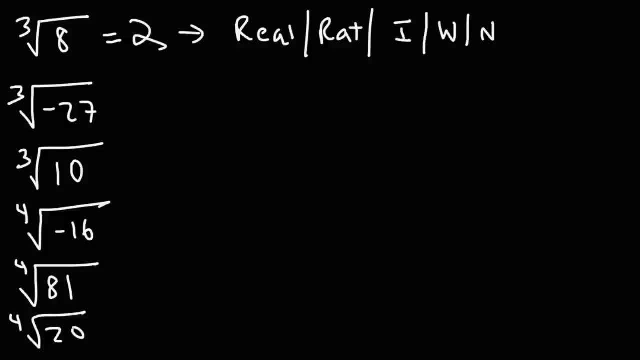 It's also a whole number and a natural number. Now, what about the cube root of negative 27? Is that real Or imaginary? Now you need to distinguish the square root of, let's say, negative 16 from the cube root of negative 27.. 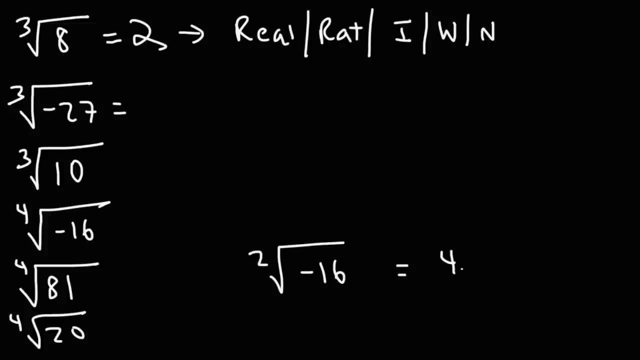 The square root of negative 16, that's not a real number, That's 4i. The square root of negative 27 is a real number, That's negative 3.. Because negative 3 times, negative 3 times, negative 3, 3 times is negative 27.. 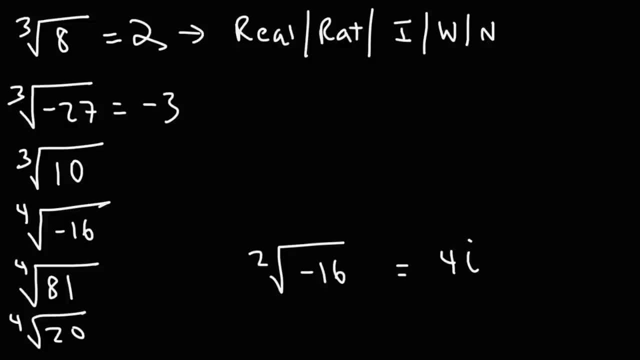 Negative 4 times negative 4 is not negative 16. It's positive 16.. So the key here is to look at the index number. If the index number is even and if you have a negative inside of it, it's going to be imaginary. 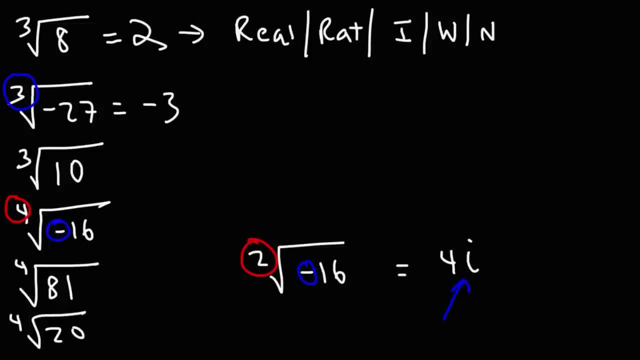 If the index number is odd, it can never be imaginary, Regardless if it's positive or negative on the inside. So that's what I want you to gather from this section of the video, So we could simplify the cube root of negative 27 to negative 16.. 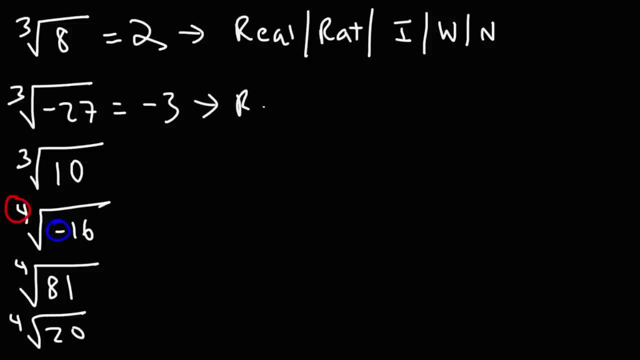 Negative 3.. Negative 3 is an integer. So that means this is going to be a real number, It's going to be rational And an integer. It's not a whole number, It's not a natural number. Now, what about the cube root of 10?? 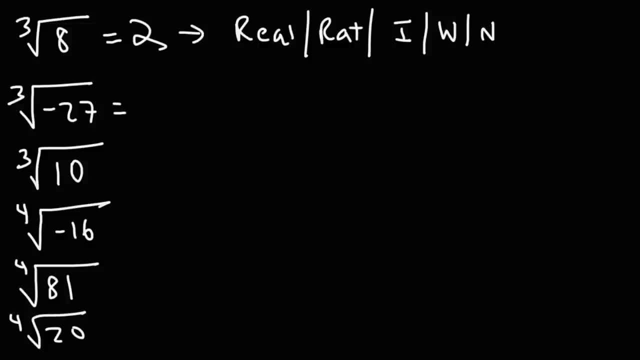 whole number and a natural number now. whole number and a natural number. now, what about the cube root of negative? what about the cube root of negative? what about the cube root of negative? now, you need to distinguish the square now. you need to distinguish the square. now. you need to distinguish the square root of, let's say, negative 16 from the. 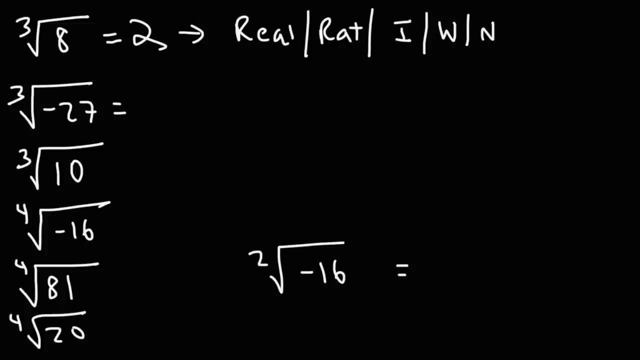 root of, let's say, negative 16. from the root of, let's say negative 16. from the cube root of negative 27: the square root cube root of negative 27, the square root cube root of negative 27, the square root of negative 16. that's not a real number. 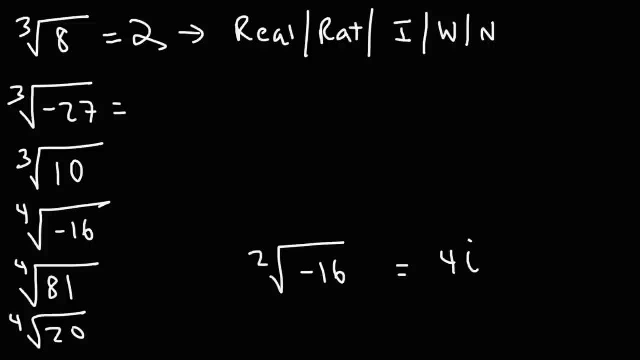 of negative 16. that's not a real number of negative 16. that's not a real number. that's 4i, the square root of negative 27. that's 4i. the square root of negative 27. that's 4i. the square root of negative 27 is a real number that's negative 3. 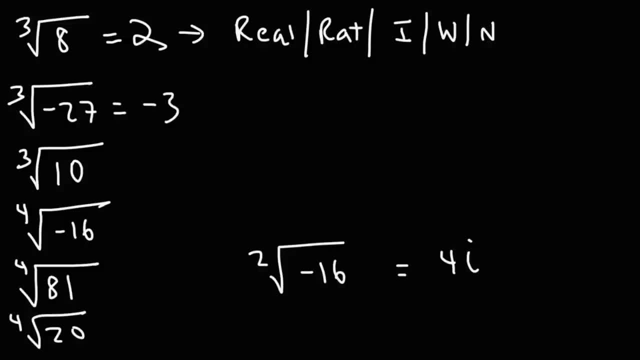 is a real number that's negative: 3 is a real number that's negative: 3 because negative 3 times. negative 3 times. because negative 3 times. negative 3 times. because negative 3 times. negative 3 times. negative 3: 3 times is negative 27. 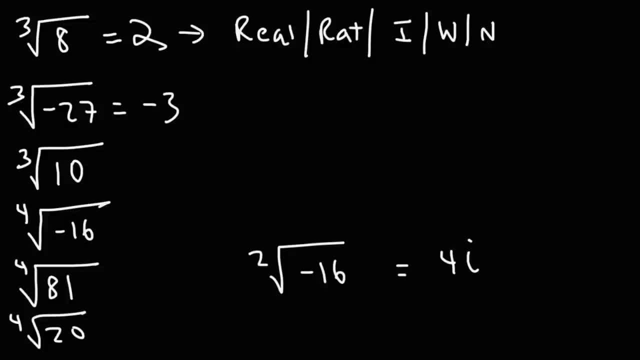 negative 3 times negative. 27 negative 3 times negative. 27 negative 4 times negative. 4 is not negative. negative 4 times negative. 4 is not negative. negative 4 times negative. 4 is not negative 16, it's positive 16. so the key: 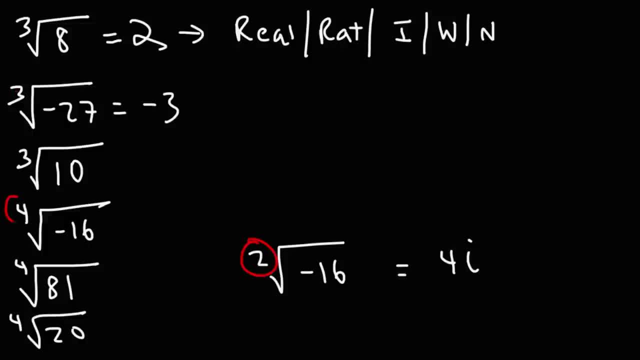 16, it's positive 16. so the key: 16, it's positive 16. so the key here is to look at the index number. if the here is to look at the index number, if the here is to look at the index number, if the index number is even and if you have. 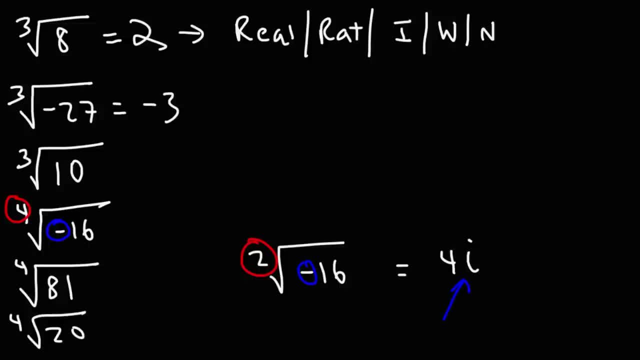 index number is even and if you have index, number is even and if you have a negative inside of it, it's going to be a negative inside of it. it's going to be a negative inside of it. it's going to be imaginary if the index number is odd. it. 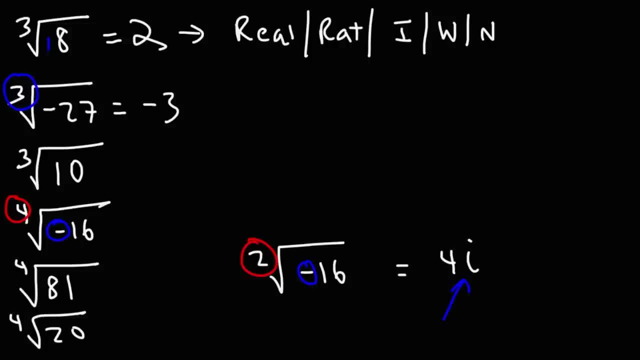 imaginary if the index number is odd. it imaginary if the index number is odd. it can never be imaginary. regardless. if can never be imaginary regardless, if can never be imaginary, regardless if it's positive or negative on the inside, it's positive or negative on the inside, it's positive or negative on the inside. so that's what I want you to gather from. 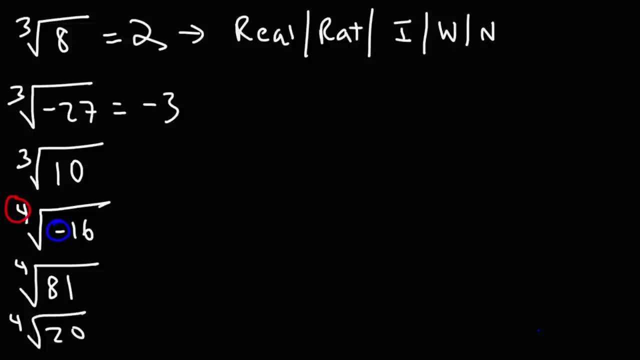 so that's what I want you to gather from, so that's what I want you to gather from this section of the video. so we could this section of the video, so we could this section of the video, so we could simplify the cube root of negative 27 to. 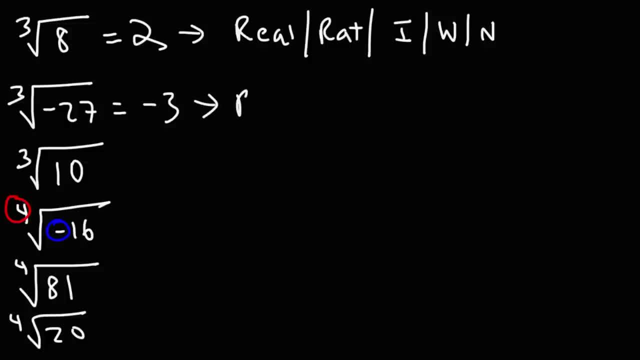 simplify the cube root of negative 27. to simplify the cube root of negative 27 to negative 3. negative 3 is an integer, so negative 3 is an integer, so negative 3 is an integer. so that means this is going to be a real number. it's. 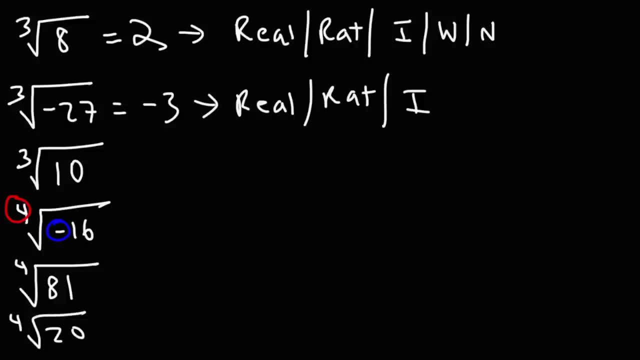 that means this is going to be a real number. it's. that means this is going to be a real number. it's going to be rational and an going to be rational and an going to be rational and an integer. it's not a whole number, it's not a. 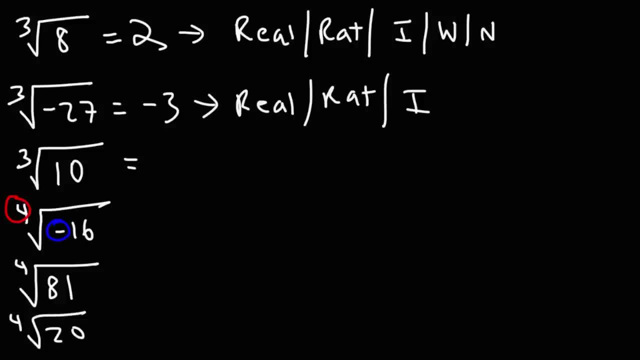 integer, it's not a whole number. it's not a integer, it's not a whole number, it's not a natural number. now, what about the natural number now? what about the natural number now? what about the cube root of 10? well, that's a positive. cube root of 10: well, that's a positive. 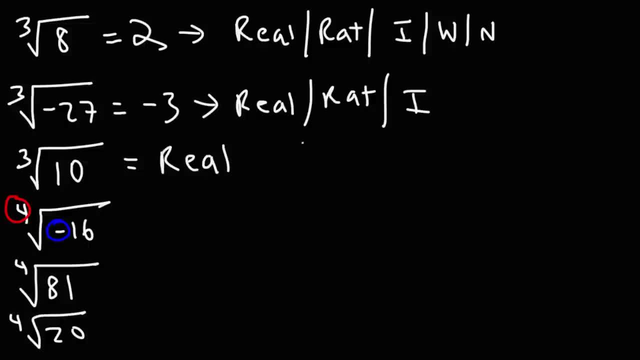 Well, that's a positive number, so it's going to be real. Is it rational or irrational? The cube root of 10 doesn't simplify into a nice integer If you type in 10 raised to the 1 third, which is equivalent to the cube root of 10,. 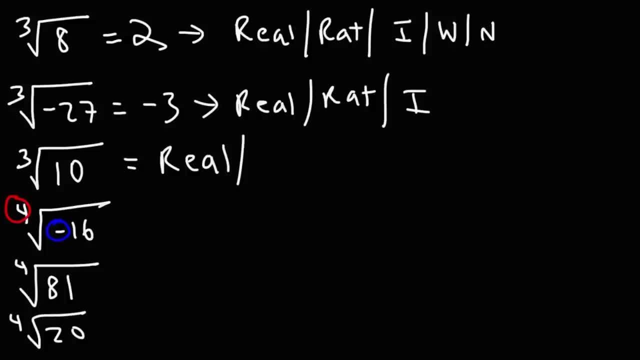 this is going to be 2.154434, and it keeps on going, So this is going to be irrational. The fourth root of negative 16.. This is, we can write this as the fourth root of 16 times the fourth root of negative 1.. 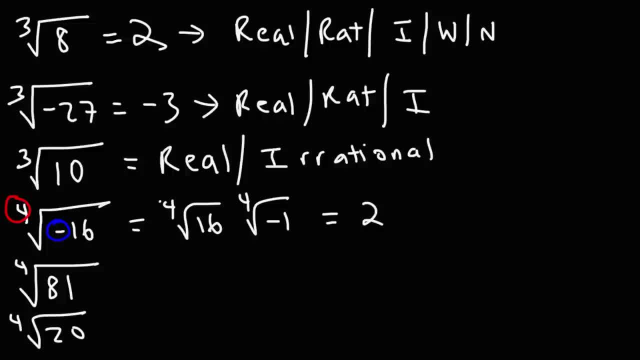 The fourth root of 16 is 2.. The fourth root of negative: 1.. Hmm, That's like taking The square root of negative 1 inside of a square root. The square root of negative 1 is i. So what we really have is the square root of i. 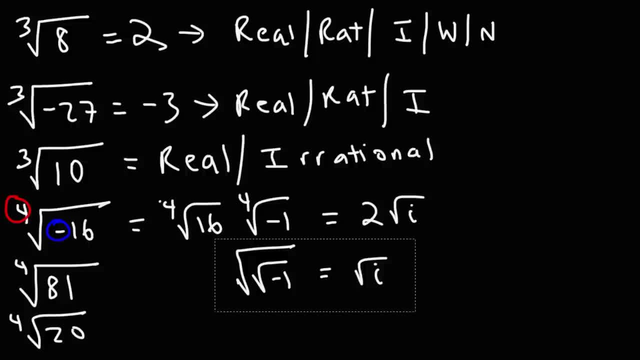 which is not going to be a real number. The fourth root of 81 is simply 3.. 3 times 3 times, 3 times 3, 4 times is 81. So that makes it real Rational. It's an integer. 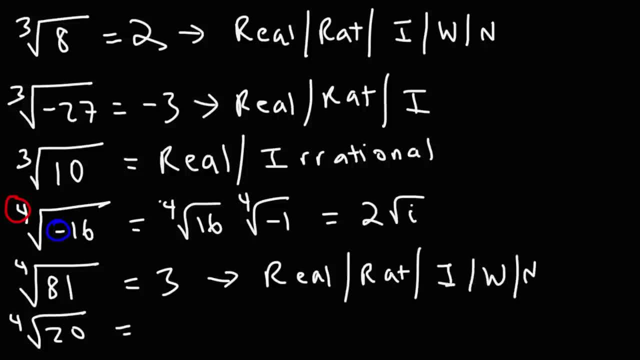 We have a whole number and a natural number: The fourth root of 20, that's 20 raised to the 1 fourth, That's 2.114742527, and I'm sure it's going to continue. So it's a real number, but it's an irrational number. 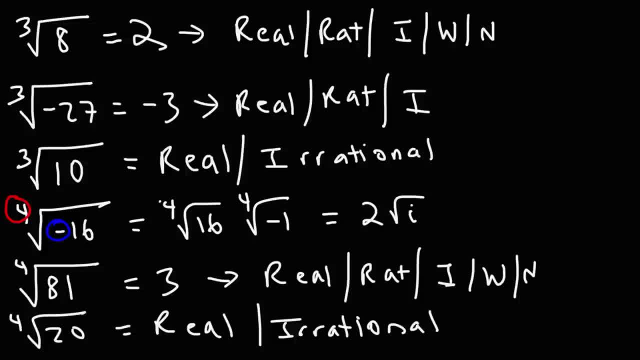 So when dealing with square roots, cube roots, fourth roots, if it doesn't simplify to a nice number, chances are it's going to be real and irrational If you have a negative number on the inside and you're dealing with an even index number. 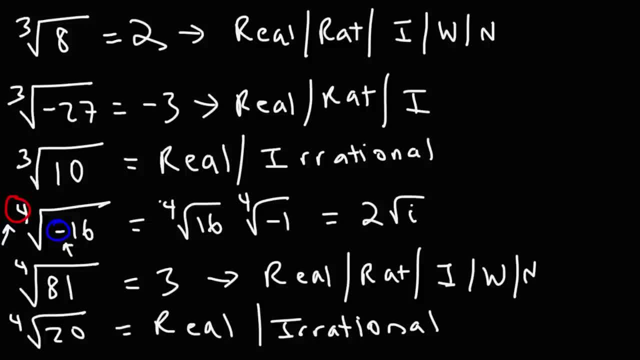 chances are it's going to be imaginary, But if it simplifies to a nice number, then you know it's going to be real and rational. So that's it for this video. Hopefully I gave you a good introduction into real numbers. 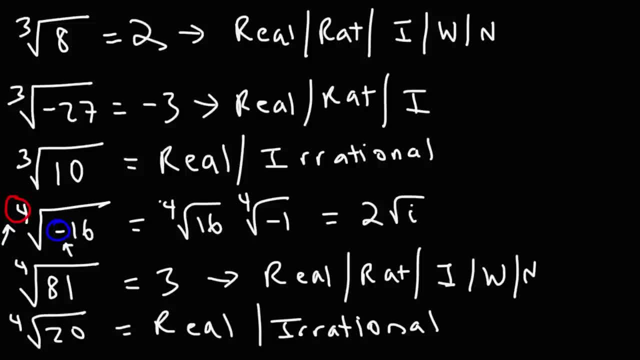 including imaginary numbers, whole numbers, integers, natural numbers, rational and irrational numbers. Thanks for watching. 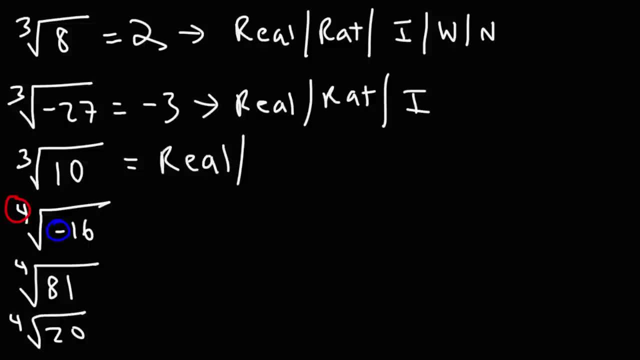 cube root of 10. well, that's a positive number, so it's gonna be real. is number, so it's gonna be real. is number, so it's gonna be real. is irrational or irrational the cube root irrational or irrational? the cube root irrational or irrational? the cube root of 10 doesn't simplify into a nice. 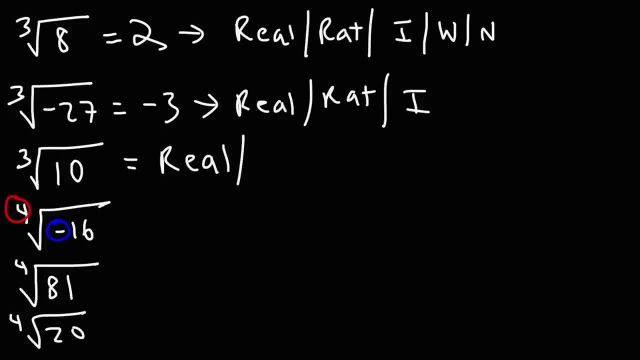 of 10 doesn't simplify into a nice of 10 doesn't simplify into a nice integer. if you type in 10 raised to the integer, if you type in 10 raised to the integer, if you type in 10 raised to the 1, 3rd, which is equivalent to the cube. 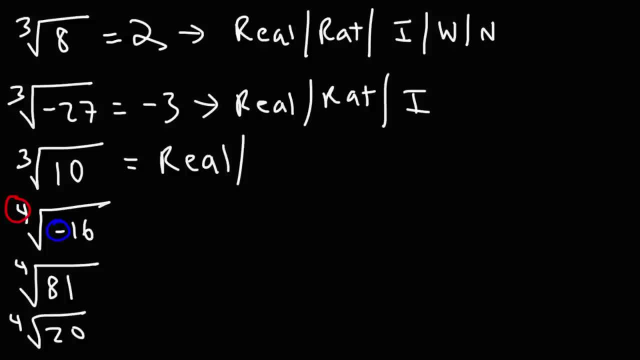 integer. if you type in 10 raised to the cube root of 10, this is going to be 2.15 root of 10. this is going to be 2.15 root of 10. this is going to be 2.15, 4, 4, 3, 4, and it keeps on going. so this is. 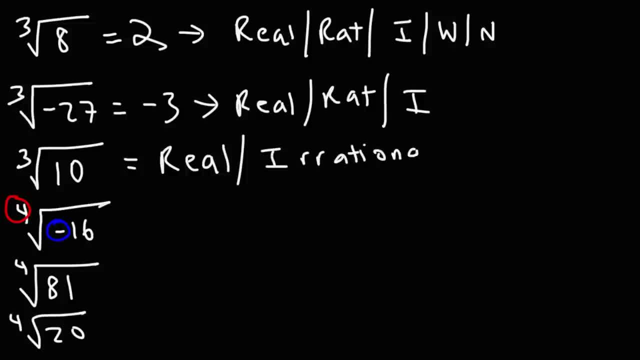 4, 4, 3, 4 and it keeps on going. so this is 4, 4, 3, 4 and it keeps on going. so this is going to be irrational, the fourth root going to be irrational, the fourth root going to be irrational, the fourth root of negative 16. this is: we can write this: 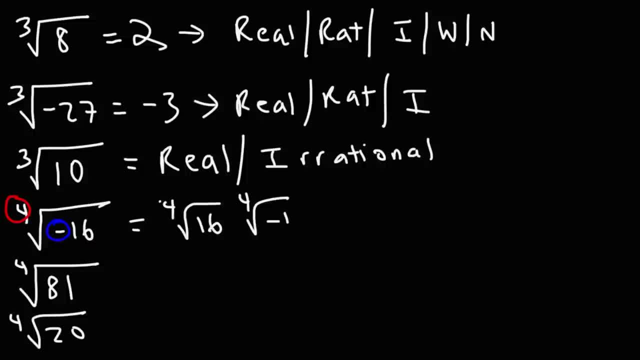 of negative 16. this is- we can write this- of negative 16. this is: we can write this: as the fourth root of 16 times the. as the fourth root of 16 times the. as the fourth root of 16 times the fourth root of negative 1: the fourth. fourth root of negative 1. the fourth fourth root of negative 1. the fourth root of 16 is 2. the fourth root of root of 16 is 2. the fourth root of root of 16 is 2. the fourth root of negative: 1. hmm, that's like taking the. 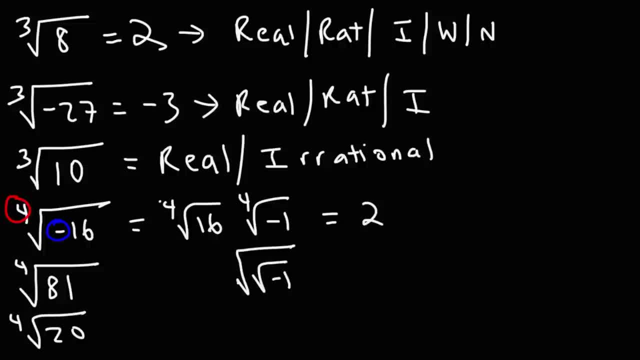 negative 1. hmm, that's like taking the negative 1. hmm, that's like taking the square root of negative 1 inside of a square root of negative. 1 inside of a square root of negative 1 inside of a square root, the square root of negative. 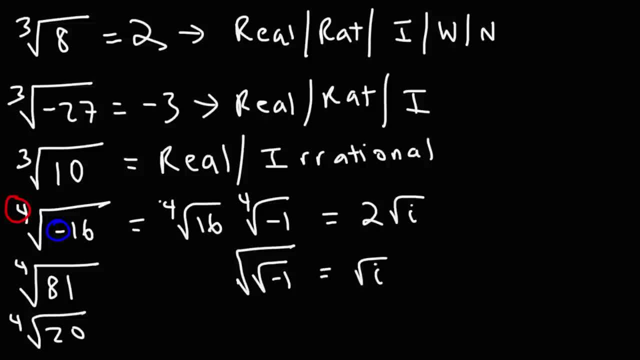 square root, the square root of negative square root, the square root of negative: 1 is I. so what we really have is the 1 is I. so what we really have is the 1 is I. so what we really have is the square root of I, which is not going to be. 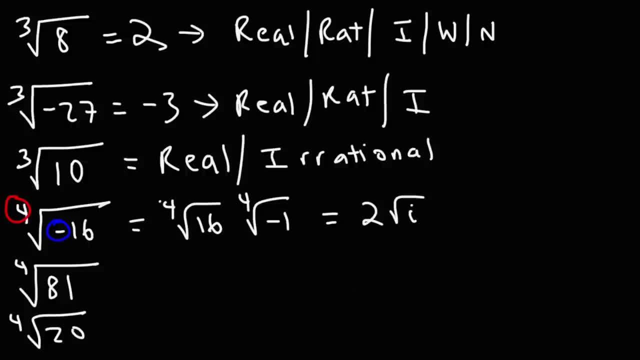 square root of I, which is not going to be square root of I, which is not going to be a real number. the fourth root of 81 is a real number. the fourth root of 81 is a real number. the fourth root of 81 is simply 3, 3 times 3 times 3 times 3, 4. 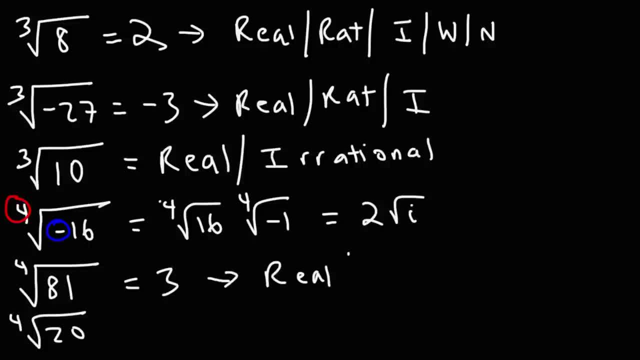 simply 3, 3 times 3 times 3 times 3. 4. simply 3, 3 times 3 times 3. 4 times is 81. so that makes it real rational. times is 81. so that makes it real rational. times is 81. so that makes it real rational. it's an integer. we have a whole number. 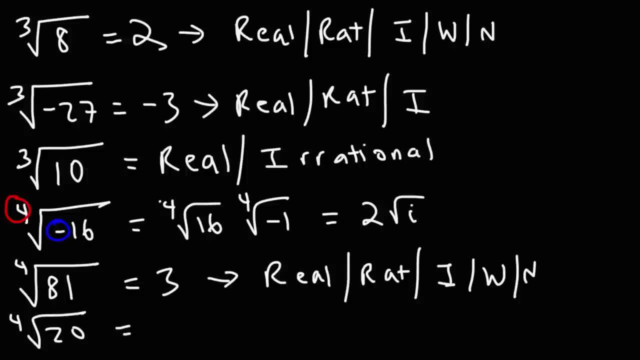 it's an integer. we have a whole number. it's an integer. we have a whole number and a natural number, the fourth root of, and a natural number, the fourth root of, and a natural number, the fourth root of 20, that's 20 raised to the 1, 4th, that's. 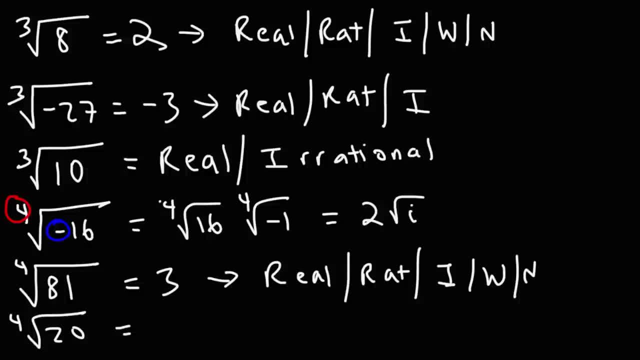 20, that's 20 raised to the 1 4th. that's 20, that's 20 raised to the 1 4th. that's 2 point 1, 1, 4, 7, 4, 2, 5, 2, 7 and I'm sure. 2 point 1, 1, 4, 7, 4, 2, 5, 2, 7, and I'm sure 2 point 1, 1, 4, 7, 4, 2, 5, 2, 7, and I'm sure it's going to continue. so it's a real. 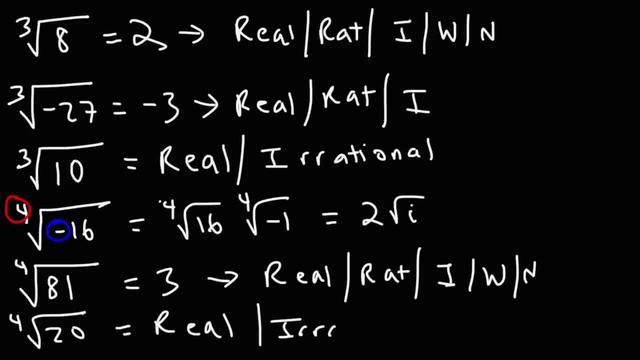 it's going to continue. so it's a real number, but it's a rational number. So when dealing with square roots, cube roots, fourth roots, if it doesn't simplify to a nice number, chances are it's going to be real and irrational If you have a negative number on the inside.